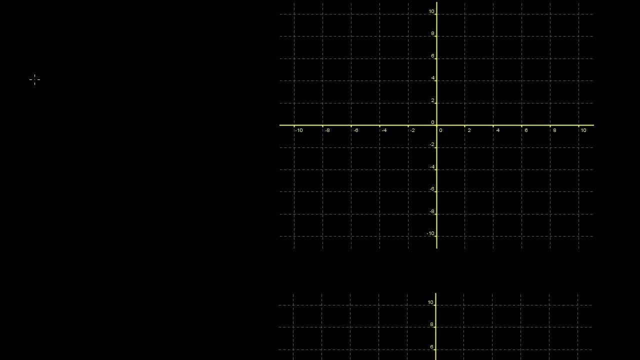 Everything we've been doing in linear algebra so far. you might be thinking it's kind of a more painful way of doing things that you already knew how to do. You've already dealt with vectors, or I'm guessing that some of you all have already dealt with vectors in your 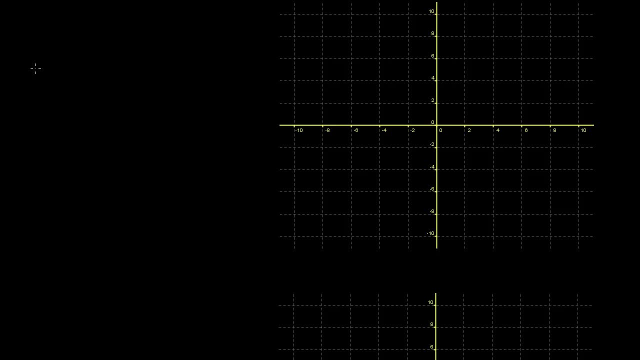 calculus or your pre-calculus or your physics classes. But in this video I hope to show you something that you're going to do in linear algebra that you've never done before and that it would have been very hard to do had you not I. 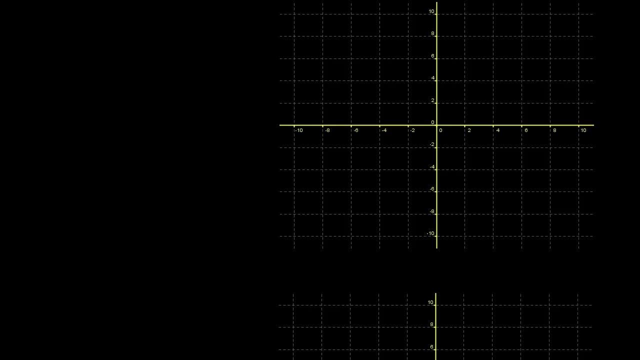 guess been exposed to these videos. Well, I'm going to start with, once again, a different way of doing something you already know how to do, So let me just define some vector here. Instead of making them bold, I'll just draw it with the. 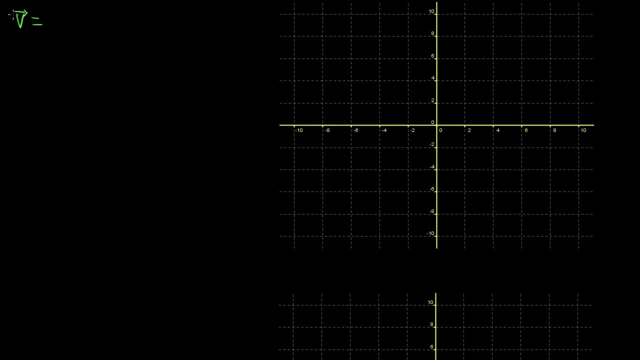 arrow on top. I'm going to define my vector to be. I could do it with the arrow on top or I could just make it super bold. I'm just going to define my vector. It's going to be a vector in R2.. 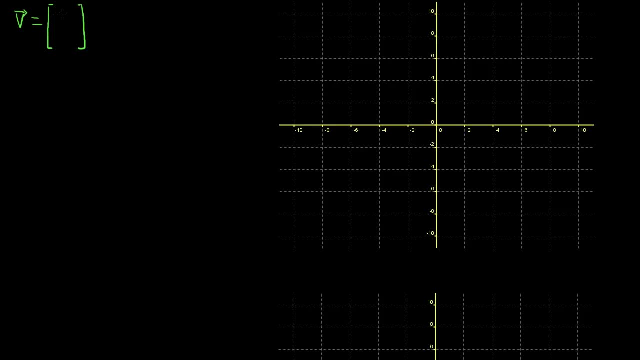 Let's just say that my vector is the vector 2, 1.. If I were to draw it in standard position it looks like this: You go 2 to the right and up 1 like that. That's my right there. that is my vector v. 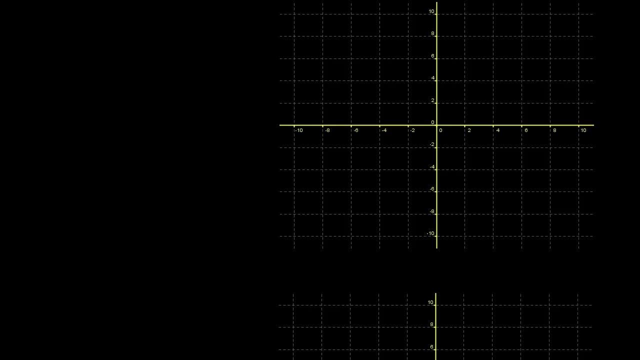 guess been exposed to these videos. Well, I'm going to start with, once again, a different way of doing something you already know how to do, So let me just define some vector here. Instead of making them bold, I'll just draw it with the. 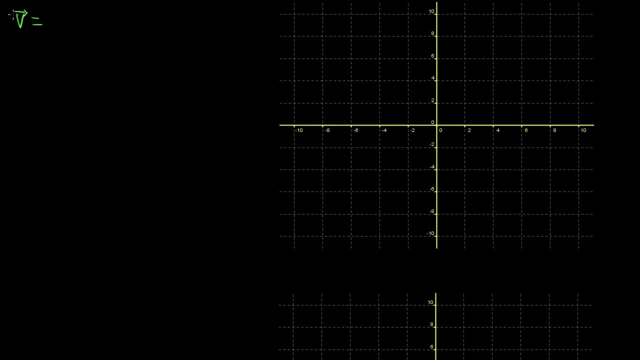 arrow on top. I'm going to define my vector to be. I could do it with the arrow on top or I could just make it super bold. I'm just going to define my vector. It's going to be a vector in R2.. 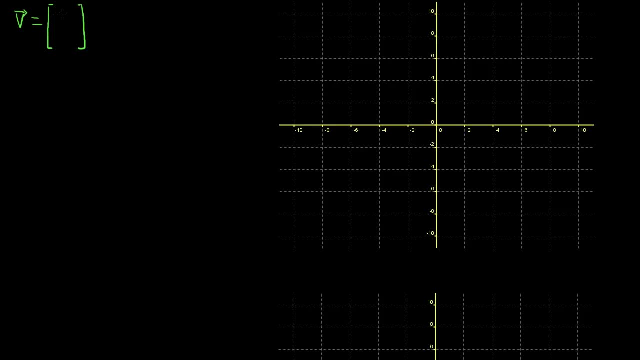 Let's just say that my vector is the vector 2, 1.. If I were to draw it in standard position it looks like this: You go 2 to the right and up 1 like that. That's my right there. that is my vector v. 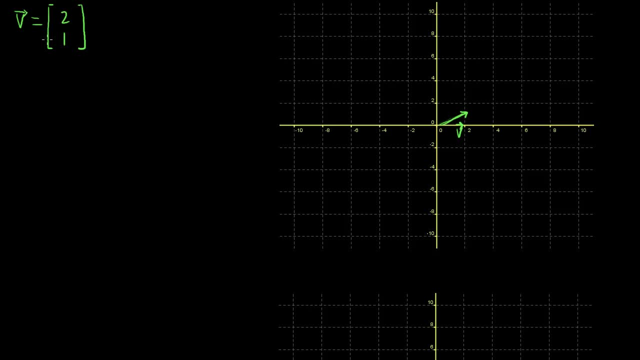 Now, if I were to ask you what are all of the possible vectors I can create? So let me define a set. Let me define a set s, and it's equal to all of the vectors I can create. if I were to multiply v times some. 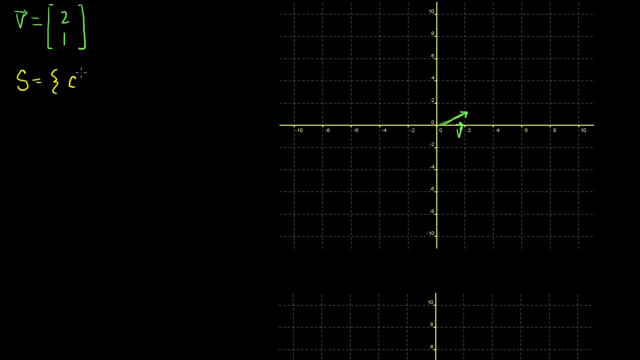 constant. so I multiply some constant, some scalar times, v times my vector v, And just to make me a little bit formal, I'm just going to say such that c is a member of the real numbers. Now, what would be a graphical representation of this set? 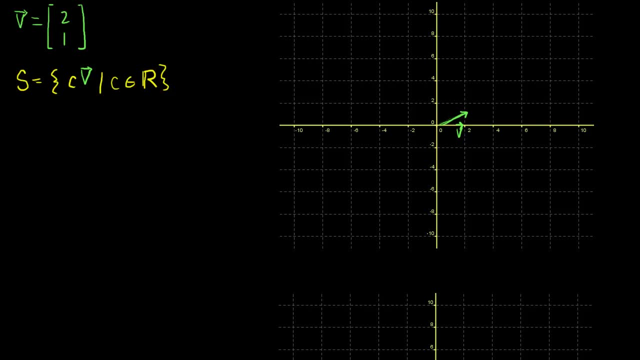 Well, if we draw them all in standard position, I mean, c could be any real number. So if I were to multiply, c could be 2.. If c is 2, c, let me do it this way: If I do 2 times our vector, I'm going to get the vector. 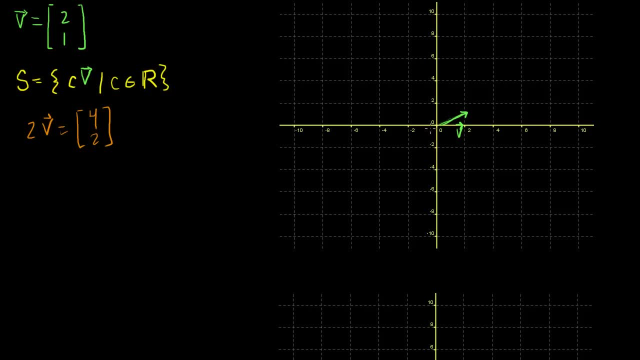 4, 2.. Let me draw that in standard position: 4, 2.. It's right there. It's this vector right there, That vector right there. It's collinear with this first vector. It's along the same line, but just goes out further too. 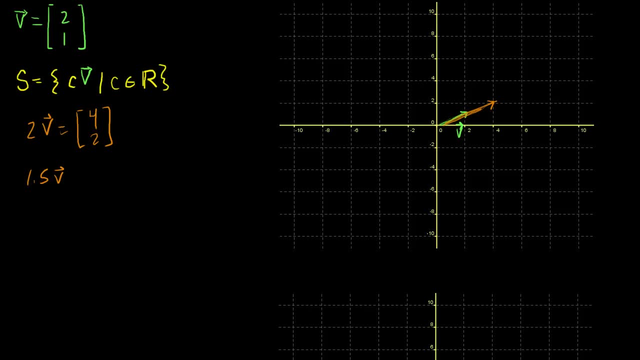 Now I could have done another. I could have done 1.5 times our vector v. Let me do that in a different color, And maybe that would be 1.5 times 2,, which is 3,, 1.5.. 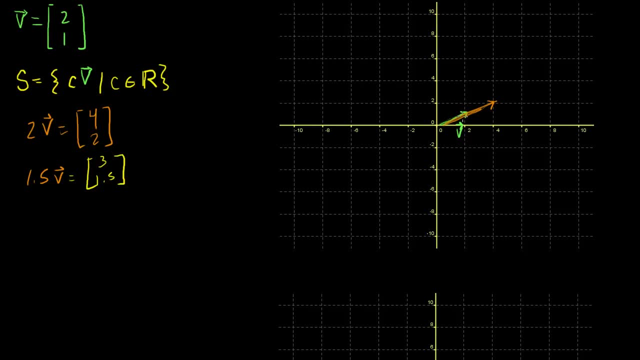 Where would that vector get me? I'd go 1.5. 1.5. 1.5., 1.5., 1.5., And then I'd go 3, and then 1.5.. I'd get right there. 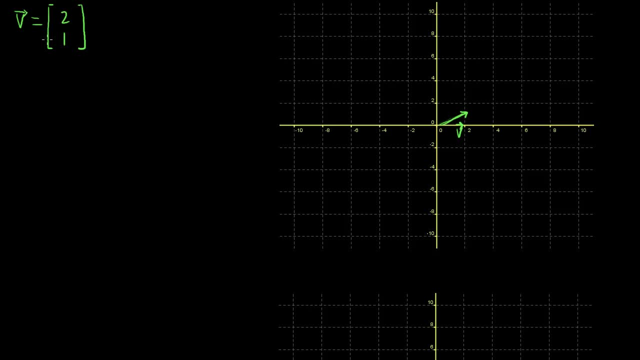 Now, if I were to ask you what are all of the possible vectors I can create? So let me define a set. Let me define a set s, and it's equal to all of the vectors I can create. if I were to multiply v times some. 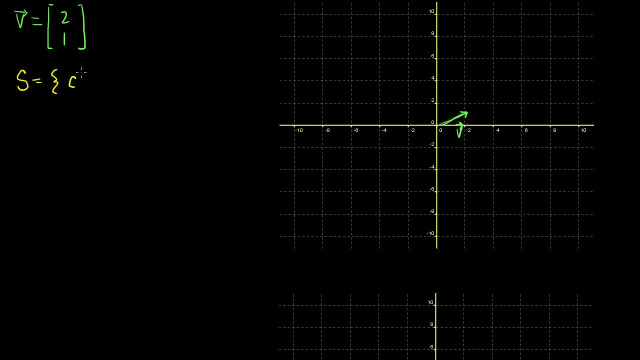 constant. so I multiply some constant, some scalar times, v times, my vector v, And just to make me a little bit formal, I'm just going to say such that c is a member and I don't want to write c is. 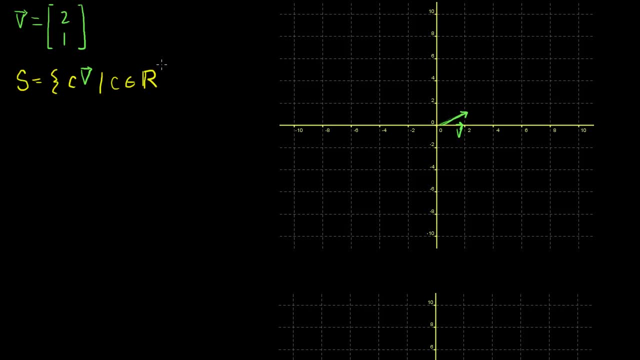 a member of the real numbers. c is a member of the real numbers. Now, what would be a graphical representation of this set? Well, if we draw them all in standard position, I mean, c could be any real number. So if I were to multiply, c could be 2.. 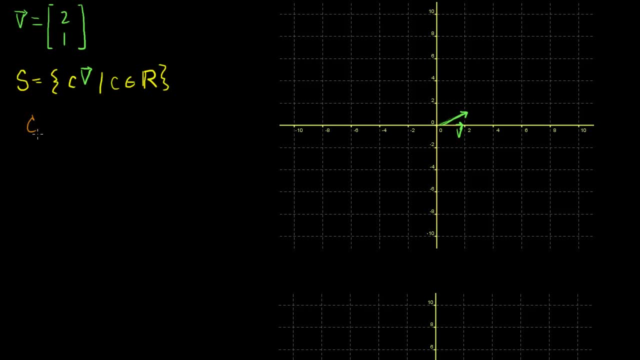 If c is 2, c, let me do it this way. If I do 2 times our vector, I'm going to get the vector v. Let me do it this way. I'm going to get the vector 4, 2.. 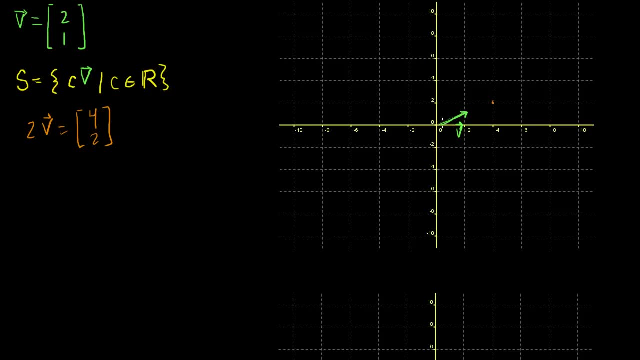 Let me draw that in standard position 4, 2.. It's right there. It's this vector right there, That vector right there. It's collinear with this first vector. It's along the same line, but it just goes out further too. 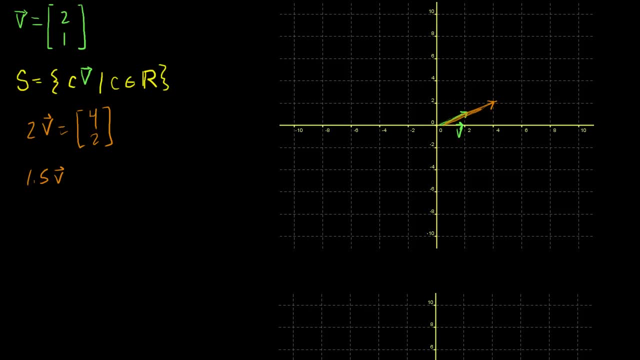 Now I could have done another. I could have done 1.5 times our vector v. Let me do that in a different color, And maybe that would be 1.5 times 2,, which is 3,, 1.5.. 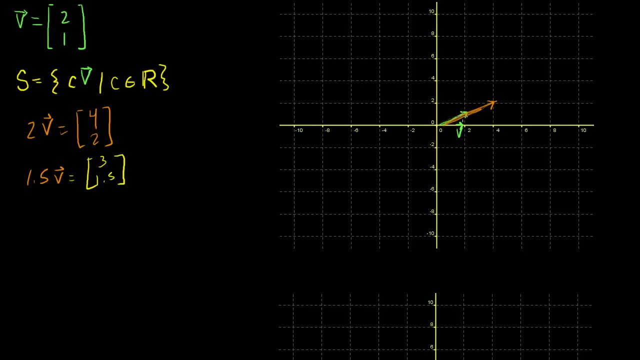 Where would that vector get me? I'd go 1.5. And then I'd go 3. And then 1.5. I'd get right there And I could multiply it by anything. I could multiply 1.4999 times vector v and get right over. 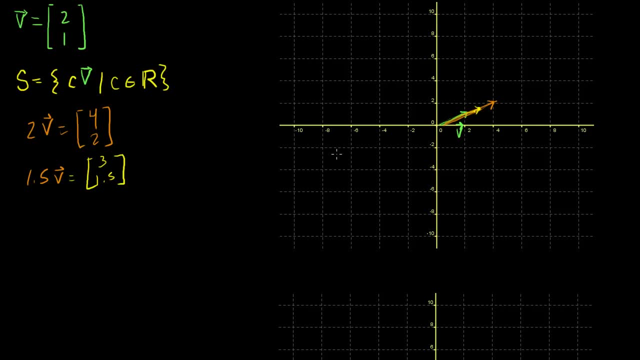 here I could do minus 0.00001 times vector v. Let me write that down. I could do 0.001 times our vector v, And where would that put me? It would put me right. little, super small vector, right. 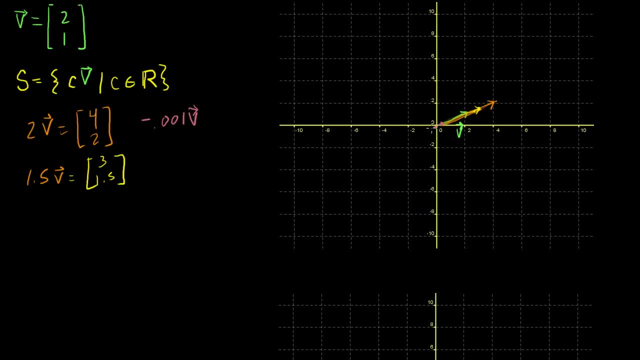 there. If I did minus 0.01, it would make a super small vector right there pointing in that direction. If I were to do minus 10, I would get a vector going in this direction. that goes way like that. Or it goes way like that. 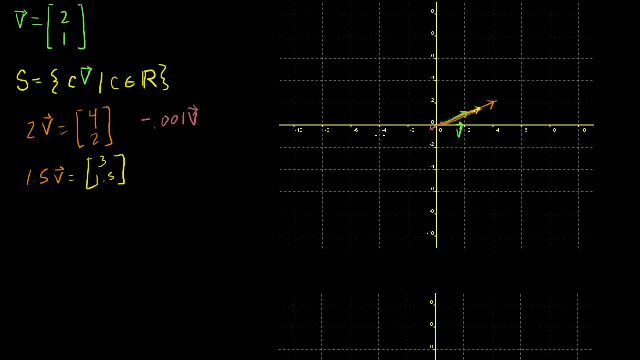 But you can imagine that if I were to plot all of the vectors in standard position- all of them that could be represented by any c in real numbers I'll essentially get. I'll end up drawing a bunch of vectors where their arrows are all. 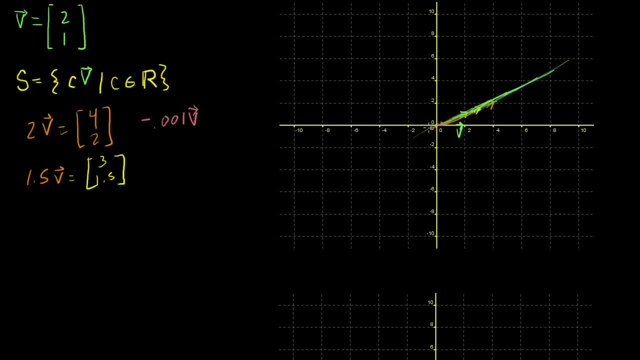 lined up along this line right there, and all lined up in even the negative direction. Let me make sure I draw it properly Along that line. like that I think you get the idea. So it's a set of collinear vectors. 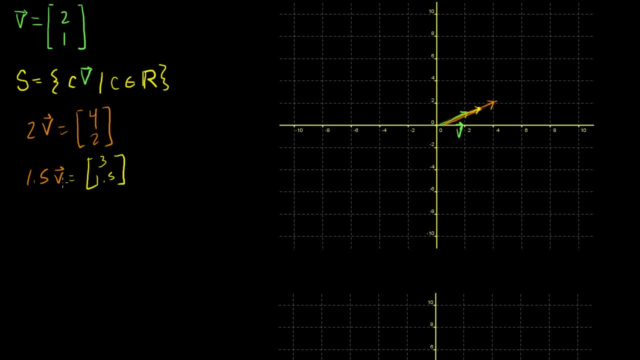 And I could multiply it by anything. I could multiply 1.4999 times vector v and get right over here. I could do minus 0.00001 times vector v. Let me write that down. I could do 0.001 times our vector v. 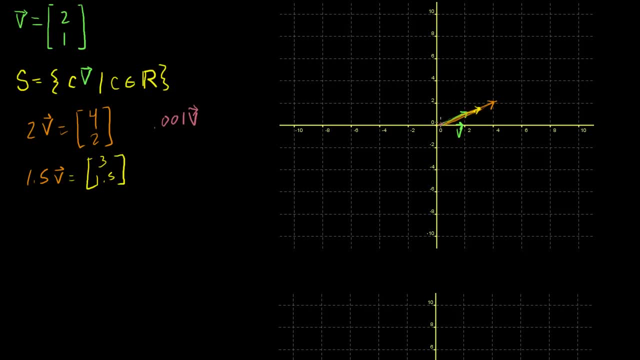 And where would that put me? It would put me right little super small vector right there. If I did minus 0.01, it would make a super small vector Right there pointing in that direction. If I were to do minus 10, I would get a vector going in. 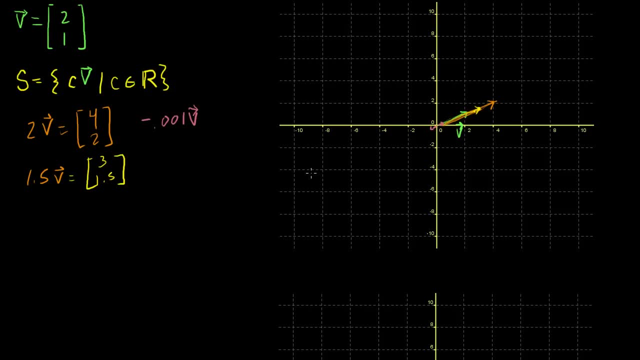 this direction. that goes way like that, Or it goes way like that. But you can imagine that if I were to plot all of the vectors in standard position- all of them that could be represented by any c in real numbers- I'll essentially get. I'll end up. 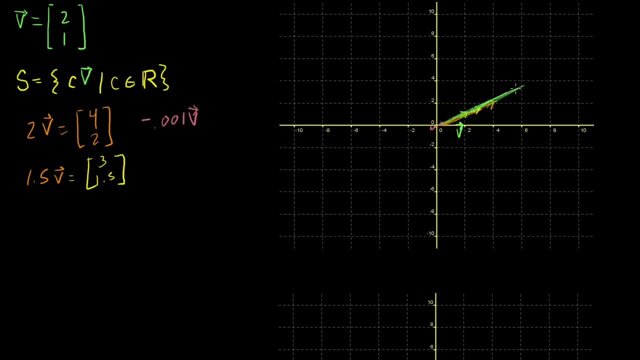 drawing a bunch of vectors where their arrows are all lined up along this line right there, and all lined up in even the negative direction. Let me make sure I draw it properly. OK, OK, OK, OK, Along that line, like that: 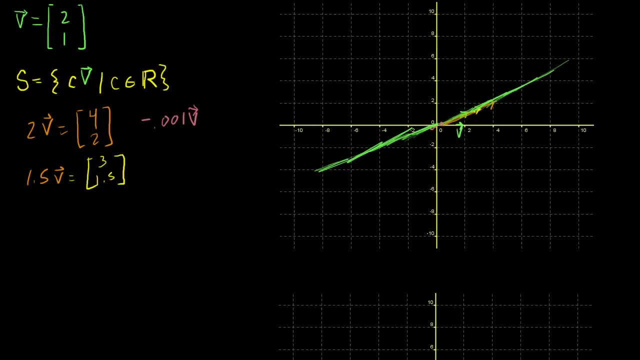 I think you get the idea. So it's a set of collinear vectors. So let me write that down. It's a set of collinear vectors And if we view these vectors as position vectors, that this vector represents a point in space in r2, this r2 is just 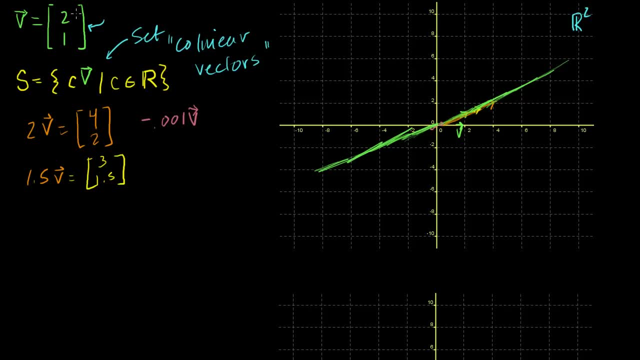 our Cartesian coordinate, Cartesian coordinate plane right here, in every direction. If we view this vector as a position vector- let me write that down as a position vector- if we view it as kind of a coordinate in r2, then this set: if we visually- 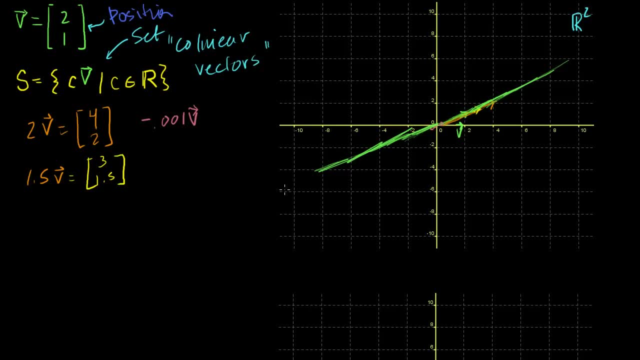 represent it as a bunch of position vectors. it'll be represented by this whole line over here. It'll be represented by this whole line over here, And I want to make that point clear because if I didn't, if it's essentially a line of slope 2, right, your rise. 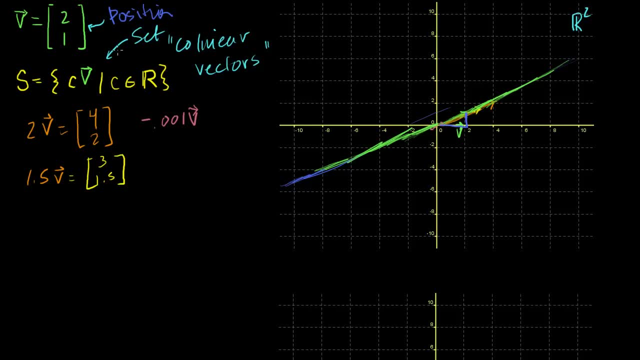 sorry, a slope 1 half. Your rise is 1.. Your rise is 1 for going over 2, but I don't want to go back to our algebra 1 notation too much. But I want to make this point that this line of slope 2, that 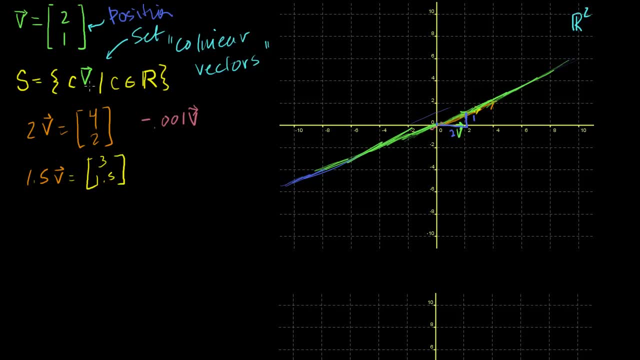 goes through the origin. this is if we draw all of the vectors in this set as in their standard form, or if we draw them all as position vectors. If I didn't make that clarification or that qualification, I could have drawn these vectors anywhere. 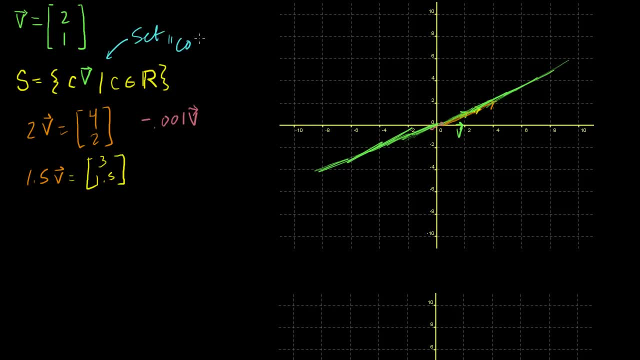 Let me write that down. It's a set of collinear vectors And if we view these vectors as position vectors, that this vector represents a point in space in r2, this r2 is just our Cartesian coordinate, It's a plane right here in every direction. 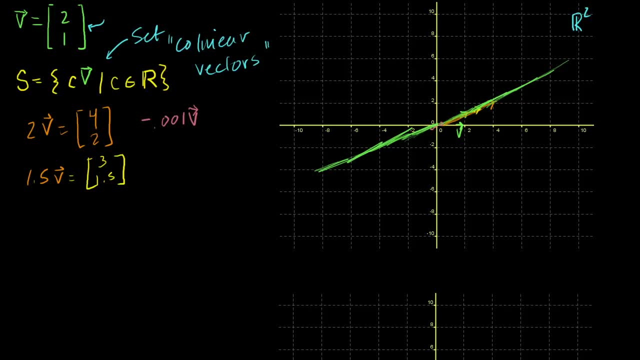 If we view this vector as a position vector- let me write that down as a position vector- if we view it as kind of a coordinate in r2, then this set, if we visually represent it as a bunch of position vectors, it'll be. 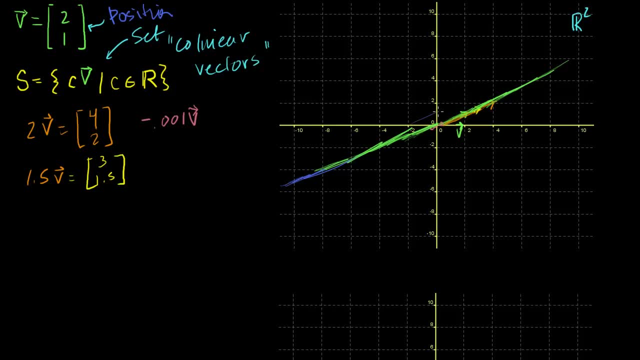 represented by this whole line over here. It'll be represented by this whole line over here, And I want to make that point clear because if I didn't, if it's essentially a line of slope 2, right, Your rise. sorry, a slope 1 half. 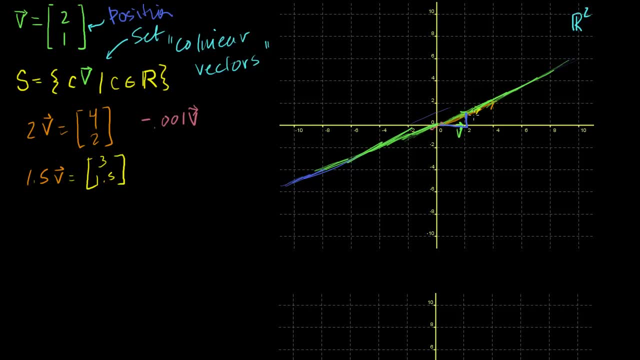 Your rise is 1.. Your rise is 1 for going over 2, but I don't want to go back to our algebra 1 notation too much. But I want to make this point that this line of slope 2 that goes through the origin. this is if we draw all of the 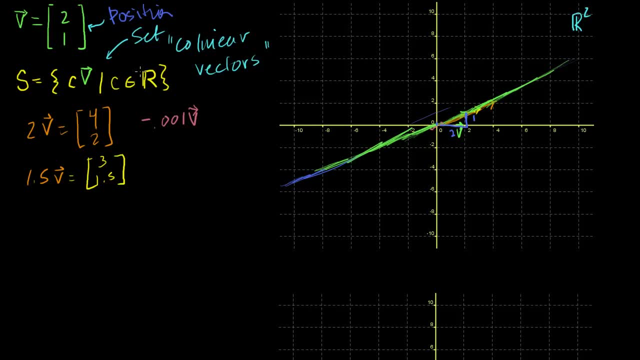 vectors in this set as in their standard form, or if we draw them all as position vectors. If I didn't make that clarification or that qualification, I could have drawn these vectors anywhere, Right, Because this 4, 2 vector I could have drawn over here. 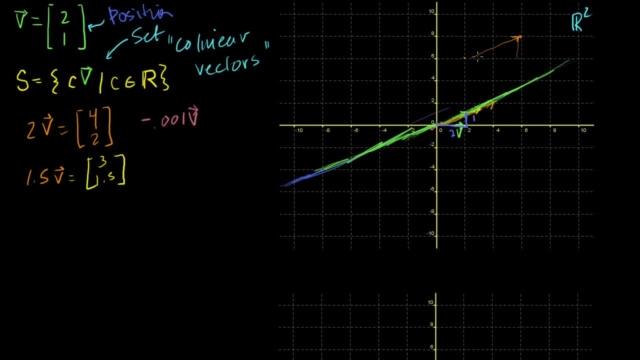 And then you know to say that it's collinear probably wouldn't have made as much visual sense to you, But I think this collinearity of it makes more sense to you if you say, oh, let's draw them all in standard form. 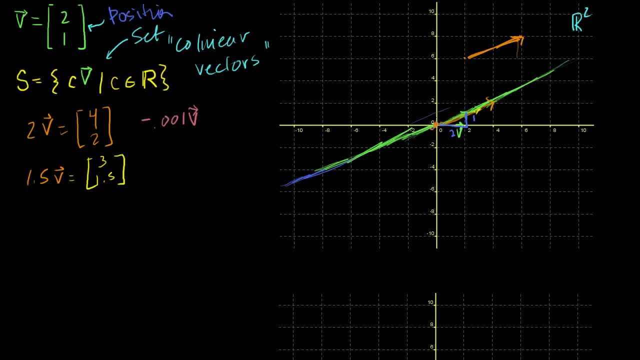 All of them start at the origin and then their tails are at the origin and their heads go essentially to the coordinate they represent. That's what I mean by their position vectors. They don't necessarily have to be position vectors, but for 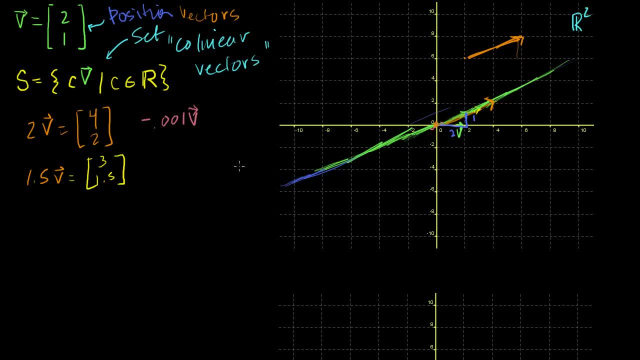 I guess the visualization in this video. let's stick to that. I was only able to represent something that goes through the origin with this slope. So you can almost view that this vector kind of represented its slope. This was. you almost want to view it as a slope vector if. 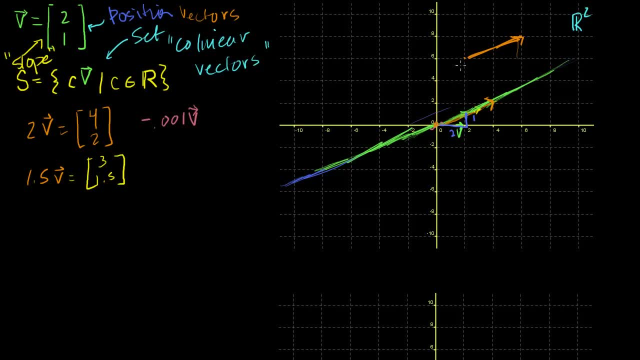 you wanted to tie it in to what you learned in Algebra 1.. What if we wanted to represent other lines that had that slope? What if we wanted to represent the line that goes the same line or, I guess, a parallel line that goes through that? 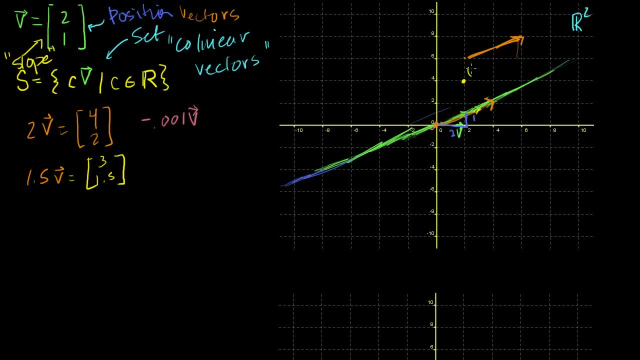 point over there, The point you know This is the point 2, comma 4.. Or if we're thinking in position vectors, we could say: that point is represented by the vector. Let me call that x. It's represented by the vector x and the vector x is. 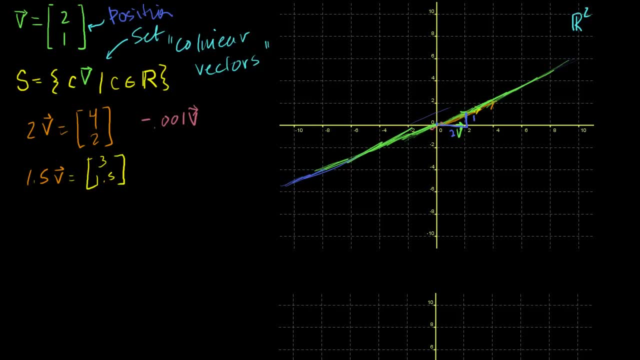 right, because I you know this 4, 2 vector I could have drawn. I could have drawn over here, And then you know to say that it's collinear. probably wouldn't have made as much visual sense to you, but I. 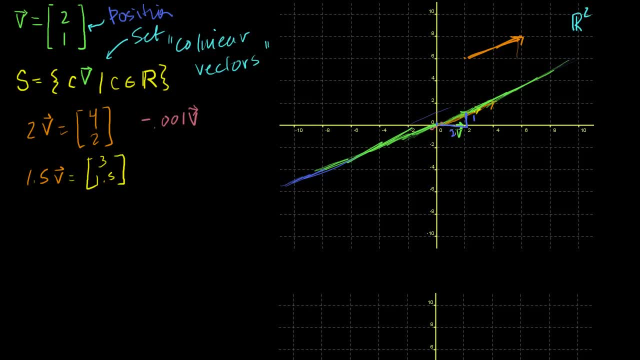 think this collinearity of it makes more sense to you if you say, oh, let's draw them all in standard form. All of them start at the origin and then their tails are at the origin and their heads go essentially to the. 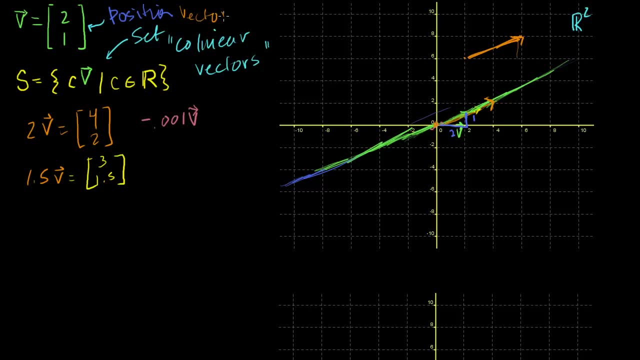 coordinate they represent. That's what I mean by their position vectors. They don't necessarily have to be position vectors, but for, I guess, the visualization in this video. well, let's stick to that. Now, I was only able to represent something that goes. 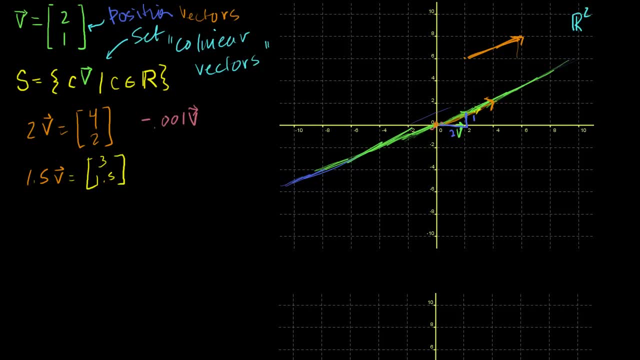 through the origin with this slope. So you can almost view that this vector kind of represented its slope. This was. you almost want to view it as a slope vector if you wanted to tie it in to what you learned in algebra 1.. What if we wanted to represent other lines that had that? 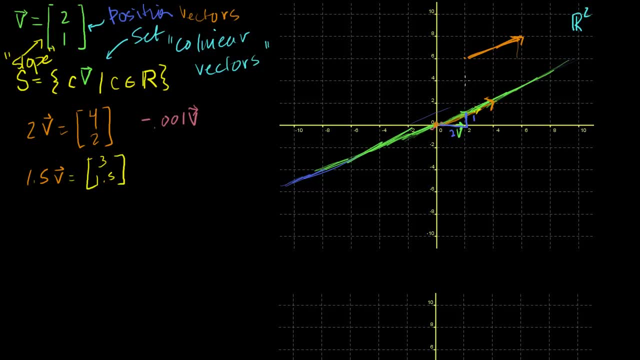 slope. What if we wanted to represent the line that goes the same line or, I guess, a parallel line that goes through that point over there, The point you know. OK, OK, OK, OK, You know. this is the point 2, comma 4.. 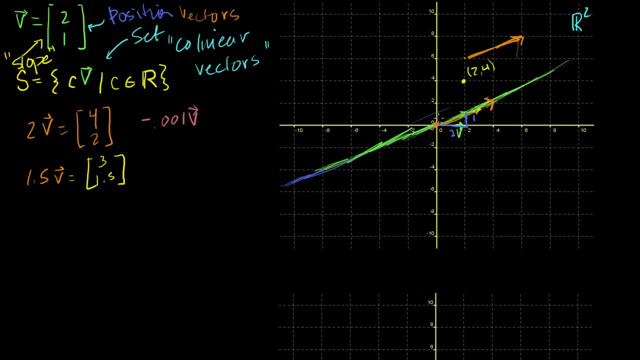 Or, if we're thinking in position vectors, we could say: that point is represented by the vector. that point is represented by the vector. let me, that point is represented by the vector. I'm going to call that x. It's represented by the vector x and the vector x is equal. 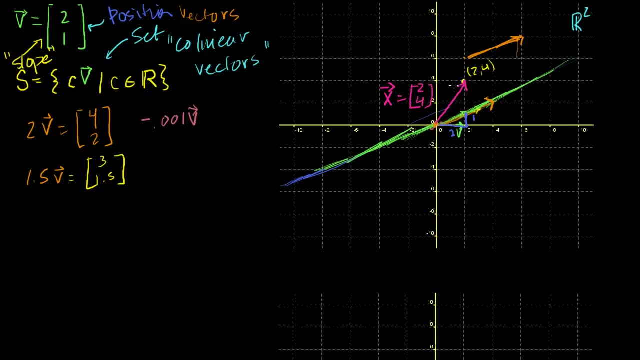 to 2, 4.. That point, right there. What if I want to represent the line that's parallel to this, that goes through that point 2, 4?? So I want to represent this line right here. I want to represent, draw it as parallel to this as I can. 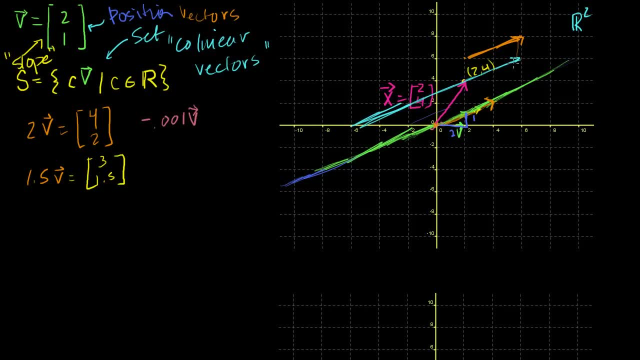 I think you get the idea. and it just keeps going like that in every direction. These two lines are parallel. How can I represent the set of all of these vectors, or the drawn in standard form, or all of the vectors that are in the 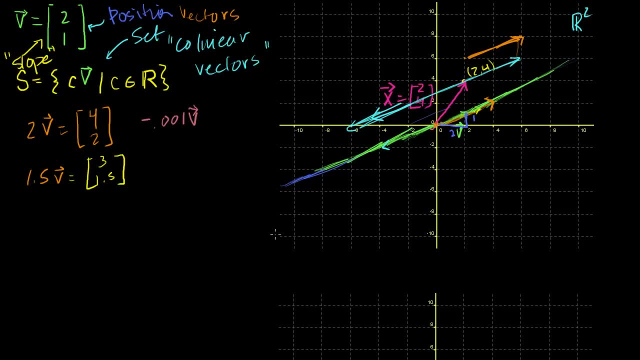 standard form, that if I were to draw them in standard form, would show this line. Well, you could think about it this way: If every one of the vectors that represented this line, if I start with any vector that was on this line and I add my 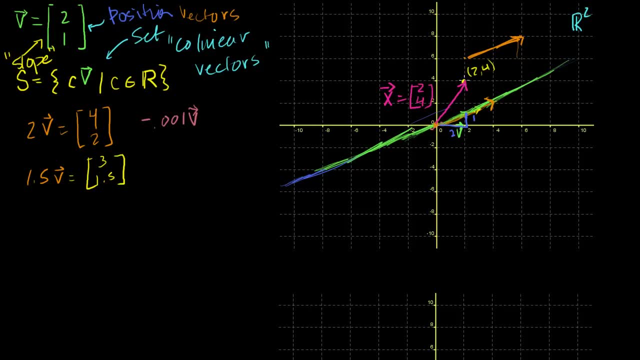 equal to 2, 4.. right there, What if I want to represent the line that's parallel to this, that goes through that point 2, 4?? So I want to represent this line right here. I want to represent, draw it as parallel to this as I can. 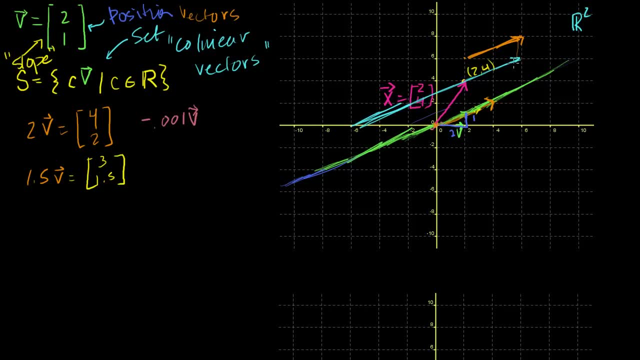 I think you get the idea. and it just keeps going like that in every direction. These two lines are parallel. How can I represent the set of all of these vectors drawn in standard form, or all of the vectors that, if I were to? 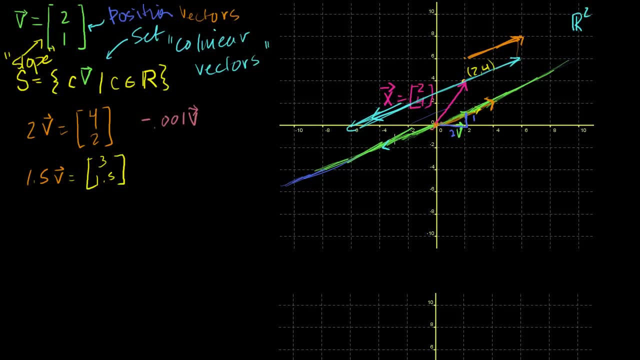 draw them in standard form, would show this line. Well, you could think about it this way: If every one of the vectors that represented this line, if I start with any vector that was on this line and I add my x vector to it, I'll show up at a corresponding point on. 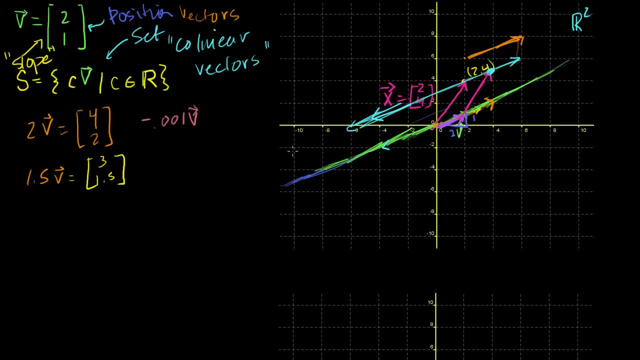 this line that I want to be at. If I start in, Let's say that this is, let's say I do, negative 2 times my original, so minus 2 times my vector v. that equaled what Minus 2, minus 4, minus 2.. 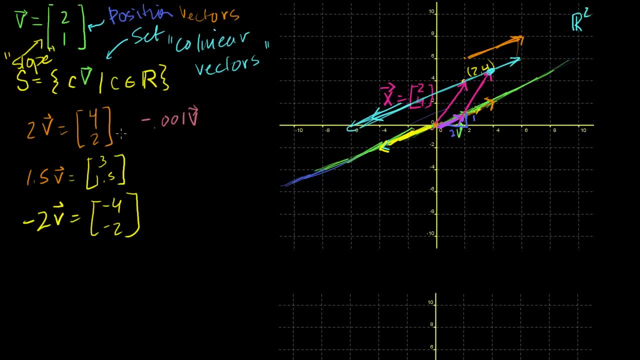 So that's that vector there. But if I were to add x to it, if I were to add my x vector, so if I were to do minus 2 times my vector v, but I were to add x to it, so plus x. 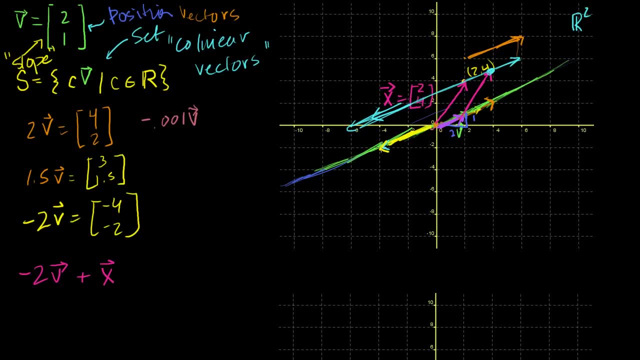 I'm adding this vector 2 comma 4 to it. So from here I'd go right to and up 4. So I'd go here. Or visually you could just say: heads to tails, so I would go right there. 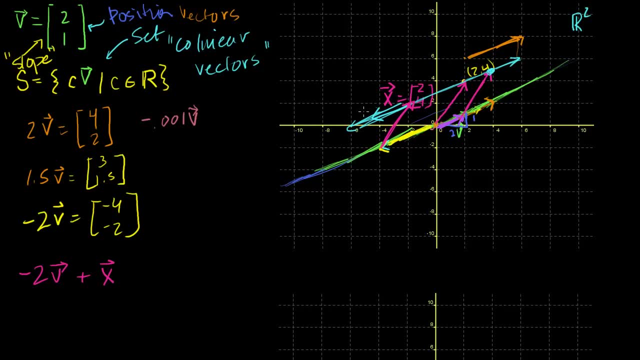 So I would end up at a corresponding point over there. I would end up at a corresponding point over there. So the set of all points. so when I define my set S as the set of all points, where I just multiply v times the scalar I, 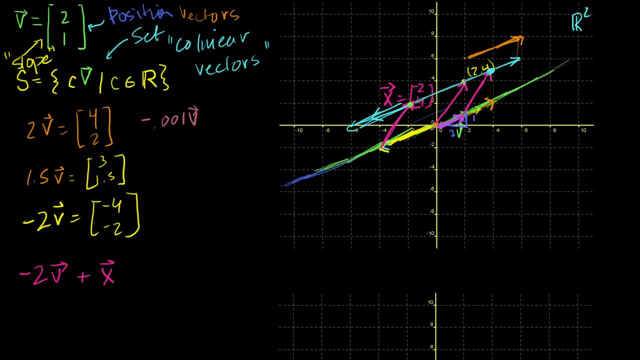 got this thing that went through the origin. But now let me define another set. Let me define a set- L, Maybe L for line. That's equal to the set of all vectors. where it's x, the vector x. I could do it bold or I'll just do an arrow on it. 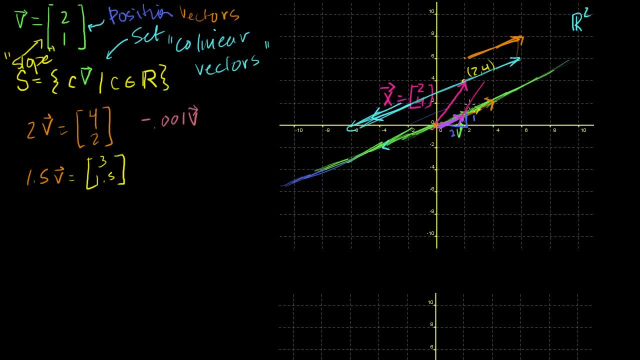 x vector to it. I'll show up at a corresponding point on this line that I want to be at. If I start, if I take, if I start, let's say that this is. let's say I was doing this. Let's do negative. let's say I do negative 2 times my original. 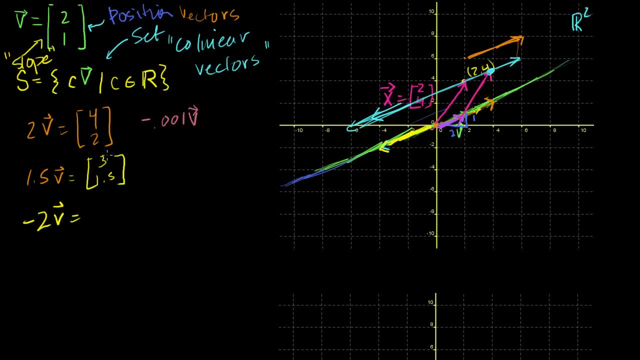 so minus 2 times my vector v, that equaled what Minus 2, minus 4, minus 2.. So that's that vector there. But if I were to add x to it, if I were to add my x vector, if 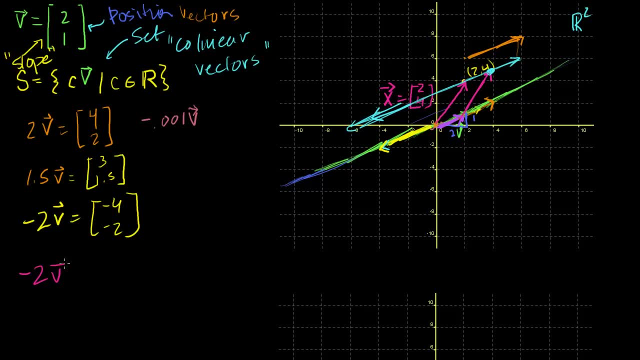 I were to add, so if I were to do minus 2 times my vector v, but I were to add x to it. so plus x, I'm adding this vector 2 comma 4 to it. So from here I'd go right to an up 4, so I'd go here. 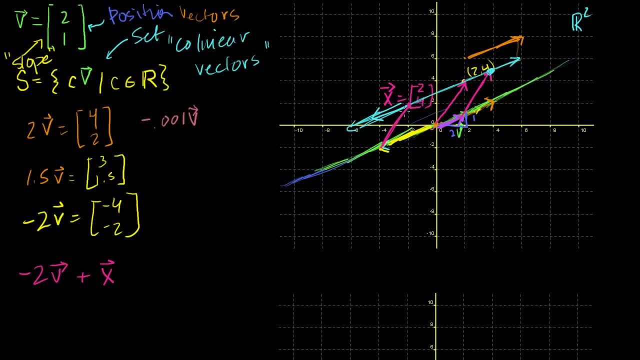 Or visually you could just say heads to tails. so I would go right there. So I would end up at a corresponding point over there. I would end up at a corresponding point over there. So the set of all points. so when I define my set S as the 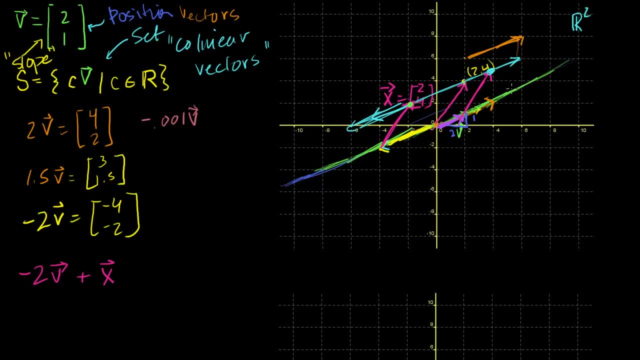 set of all points where I just multiply v times the scalar. I got this thing that went through the origin. But now let me define another set. Let me define a set L, maybe L for line. It's equal to the set of all vectors, where it's x the. 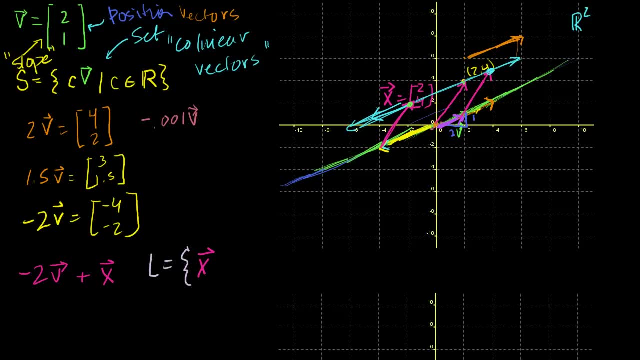 vector x. I could do it bold or I'll just do an arrow on it, plus some scalar. I could use c, but let me use t, because I'm going to call this a parametrization of the line. So, plus some scalar. t times my vector v. 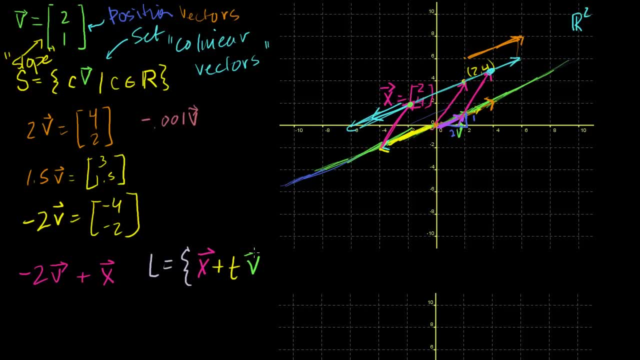 Times my vector v: Where, Where, Where, Where, Or such that t could be any member of the real numbers. So what is this going to be? This is going to be this blue line If I were to draw all of these vectors in standard position. 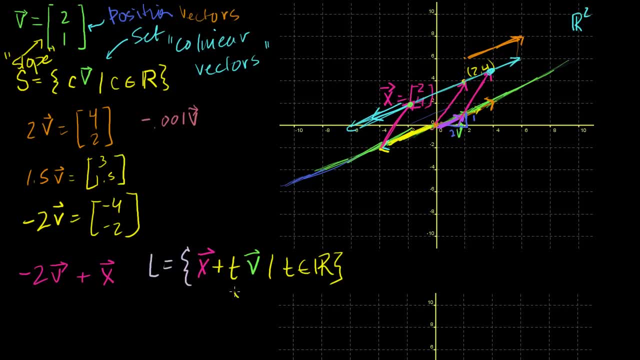 I'm going to get my blue line. For example, if I do minus 2, this is minus 2, times my vector v, I get here. Then if I add x, I go there. So the vector, this vector right here, that has its. 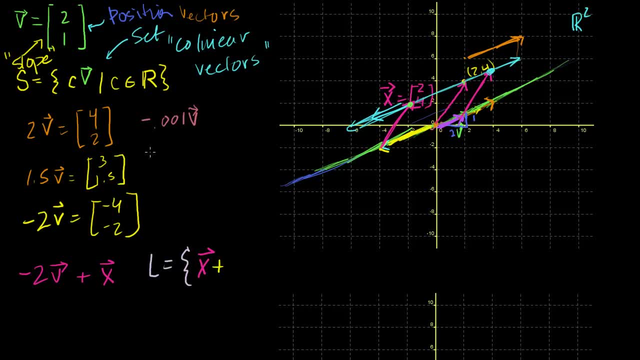 plus some scalar. I could use c, but let me use t because I'm going to call this a parametrization of the line. So, plus some scalar, t times my vector v Where or such that t could be any member of the real. 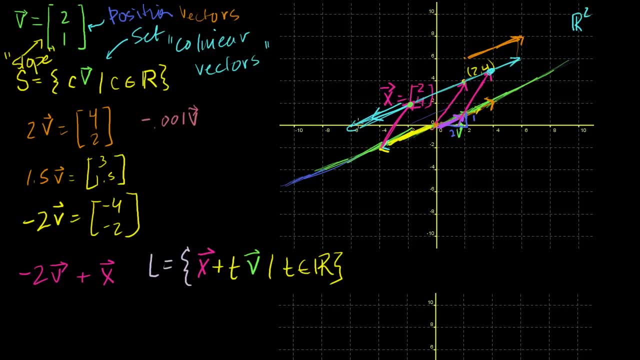 numbers. So what is this going to be? This is going to be this blue line. If I were to draw all of these vectors in standard position, I'm going to get my blue line. For example, if I do minus 2,, this is minus 2, times my. 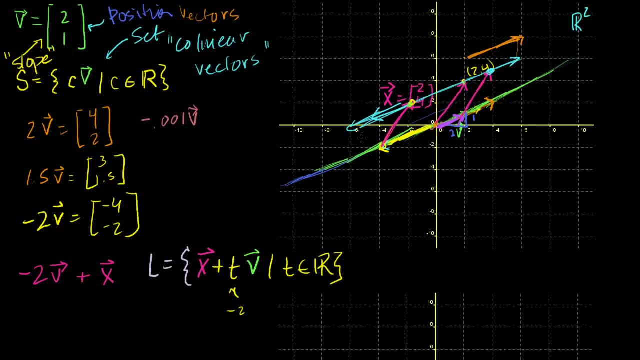 vector v, I get here, Then if I add x, I go there. So the vector, this vector right here, that has its end point right there, Its end point sits on that line. I could do that with anything If I take this vector. this is some scalar times. my vector v: 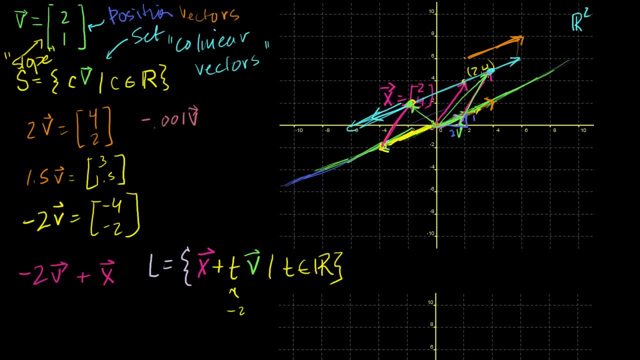 and I add x to it, I end up with this vector whose end point- if I view it as a position vector- its end point dictates some coordinate in the xy plane. So it'll be at that point, So I can get to any of these vectors. 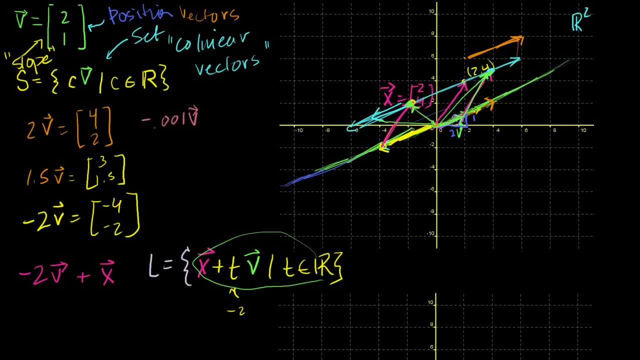 This is a set of vectors right here and all of these vectors are going to point. they're essentially going to point to something when I draw them in standard form. If I draw them in standard form, they're going to point to a point on that blue line. 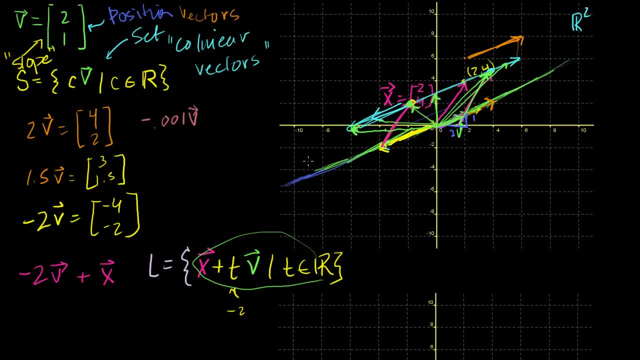 Now you might say: hey, Sal, this was a really obtuse way of defining a line. We do it in Algebra 1, where we just say: hey, y is equal to mx plus b, and we figure out the slope by figuring out the 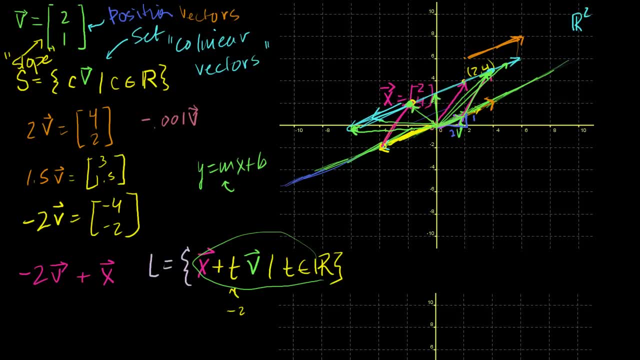 difference of two points, and then we do a little substitution And this is stuff you learned in seventh or eighth grade. This was really straightforward. Why am I defining this obtuse line? Why am I defining this obtuse line? Why am I defining this set here and making you think in? 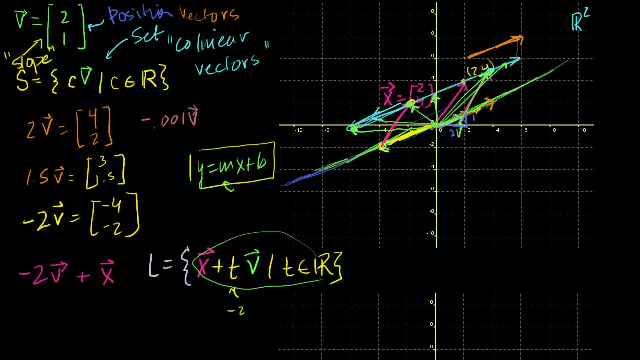 terms of sets and vectors and adding vectors, And the reason is because this is very general. This worked well in R2.. So in R2, this was great. I mean, we just have to worry about x's and y's, But what about the situation? 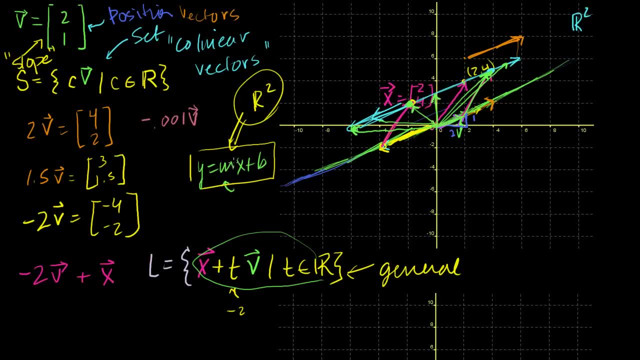 I mean notice. in your Algebra class your teacher never really told you much- or at least in the ones I took- about how do you represent lines in three dimensions. I mean, Maybe some classes go there, but they definitely didn't. 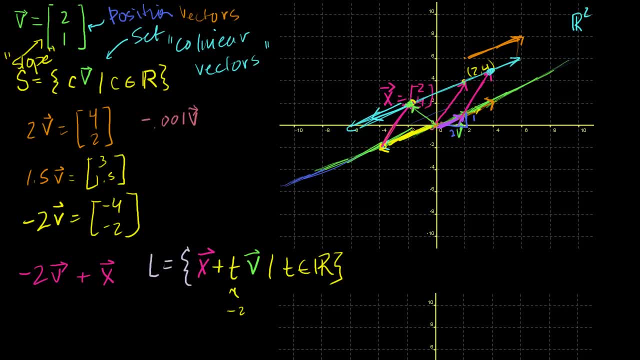 endpoint, right there. Its endpoint sits on that line. I could do that with anything. If I take this vector- this is some scalar times- my vector v and I add x to it, I end up with this vector whose endpoint- if I view it as a position vector, its endpoint. 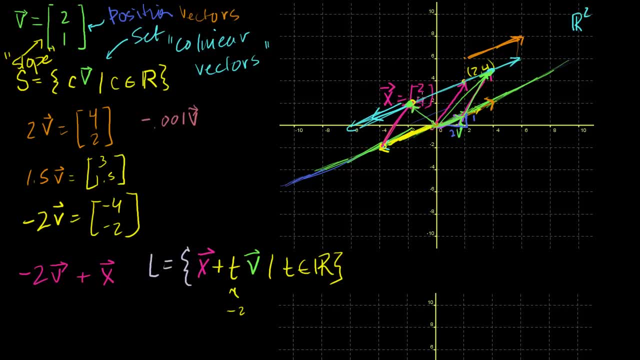 dictates some coordinate in the xy plane. So it'll be at that point. So I can get to any of these vectors. This is a set of vectors right here and all of these vectors are going to point. they're essentially going to point to: 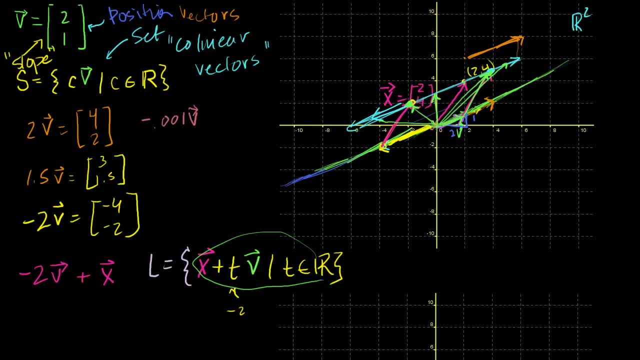 something When I draw them in standard form. if I draw them in standard form, they're going to point to a point on that blue line. Now you might say: hey, Sal, this was a really obtuse way of defining a line. 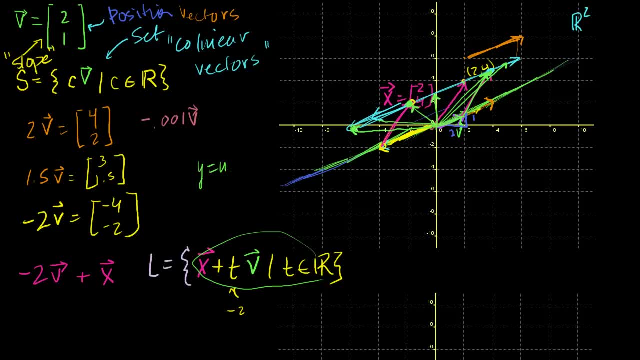 I mean we do it in Algebra 1, where we just say, hey, y is equal to mx plus b, and we figure out the slope by figuring out the difference of two points, and then we do a little substitution, And this is stuff you learned in seventh or eighth grade. 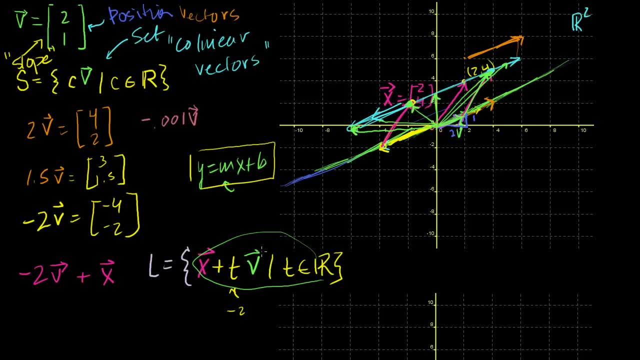 This was really straightforward. Why am I defining this obtuse set here And making you think in terms of sets and vectors and adding vectors? and the reason is because this is very general. This worked well in R2.. So in R2, this was great. 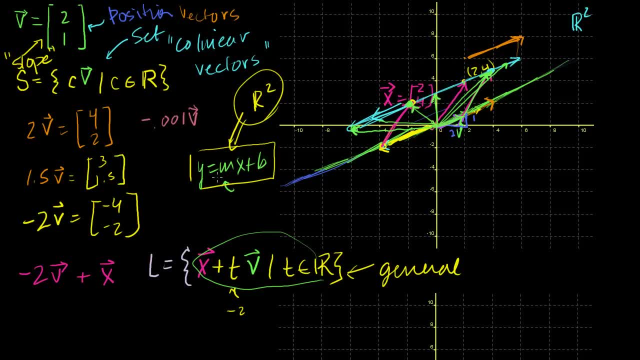 I mean we just have to worry about x's and y's, But what about the situation? I mean, notice, in your Algebra class your teacher never really told you much, or at least in the ones I took about. how do you represent lines in three dimensions? 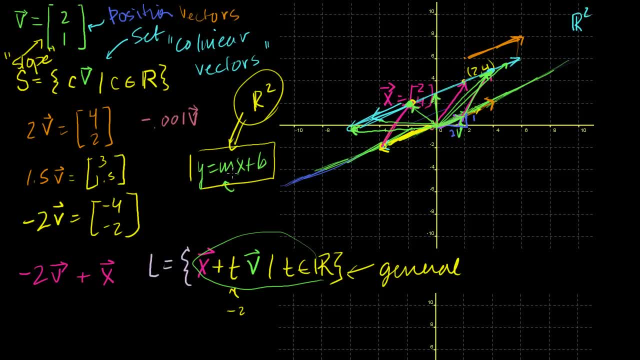 And I mean maybe some classes go there, But they definitely didn't tell you how do you represent lines in four dimensions or 100 dimensions, And that's what this is going to do for us Right here. I defined x and v as vectors in R2.. 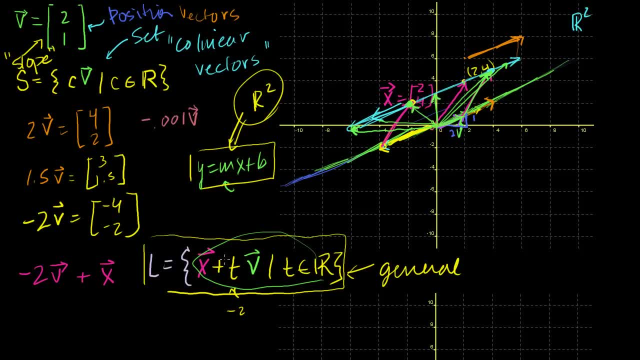 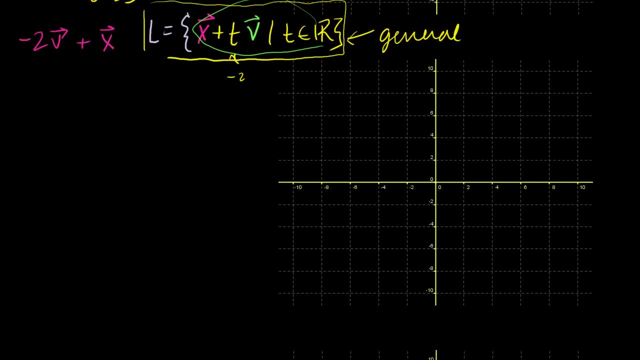 They're two-dimensional vectors, But we can extend it to an arbitrary number of dimensions. So just to kind of hit the point home, let's do one more example in R2, where it's kind of the classic algebra problem where you need to find the equation for the line. but here 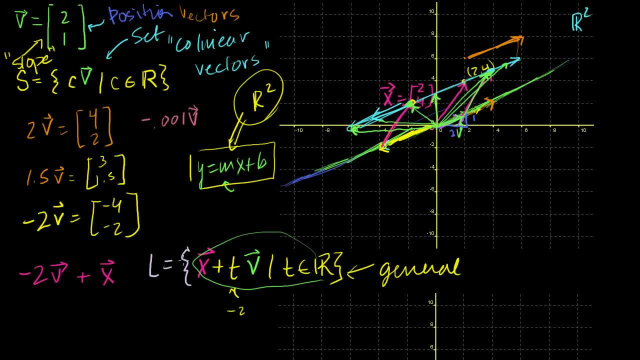 tell you how do you represent lines in four dimensions or 100 dimensions, And that's what this is going to do for us. Right here, I defined x and v as vectors in R2.. They're two-dimensional vectors, But we can extend it to an arbitrary number of. 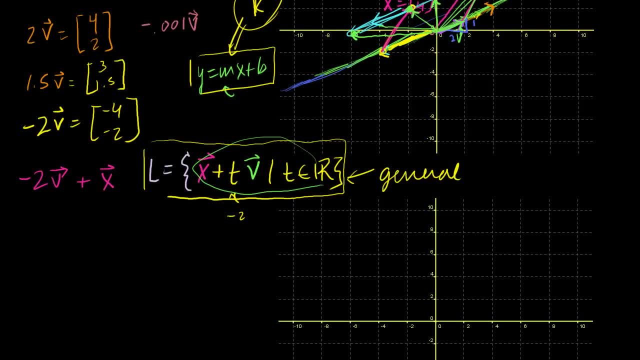 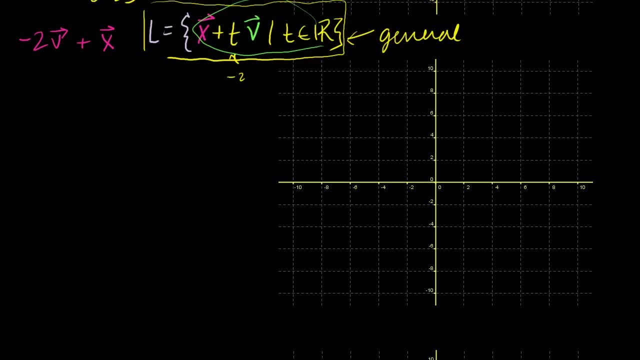 dimensions. So just to kind of hit the point home, let's do one more example in R2, where it's kind of the classic algebra problem where you need to find the equation for the line, But here we're going to call it the set. 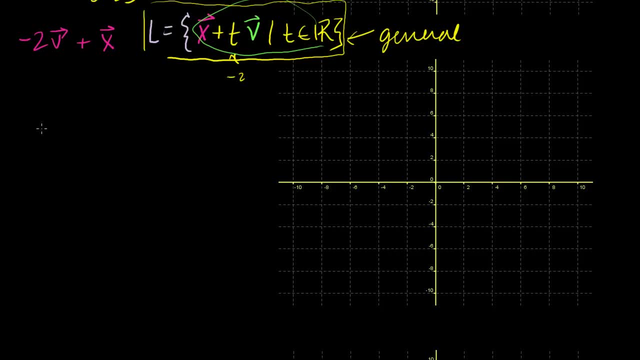 definition for the line. Let's say we have two vectors. Let's say we have the vector a, which I'll define as 2, 1.. So if I were to draw in standard form, it's 2,, 2, 1.. 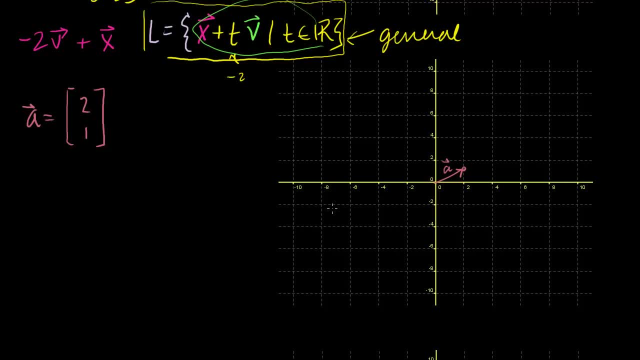 That's my vector a, right there. And let's say I have vector b. Let me define vector a. Let me define vector b. I'm going to define it as I don't know. let me define it as 0, 3.. 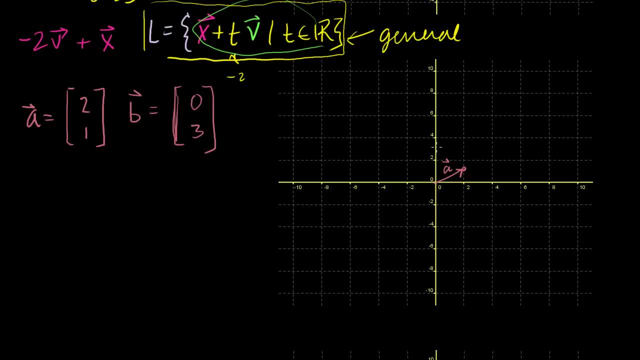 So my vector b is 0.. I don't move to the right at all And I go up, So my vector b will look like that. my vector b. Now I'm going to say that these are position vectors. We draw them in standard form. 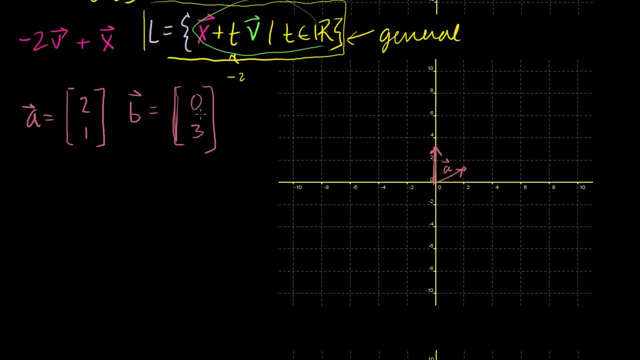 When you draw them in standard form, their endpoints represent some position, So you can almost view these as coordinate points in R2.. This is R2.. All of these coordinate axes I draw are going to be R2.. Now what if I asked you give me a parameterization of the? 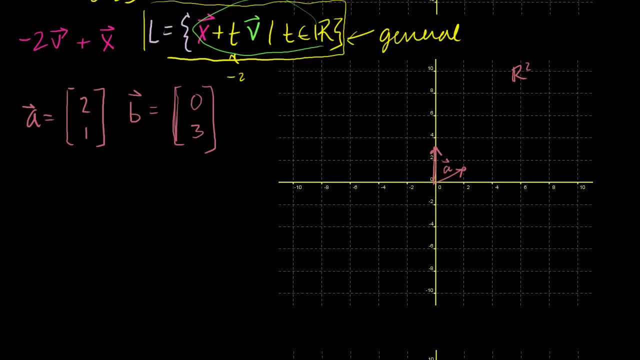 line that goes through these two points. So essentially I want the equation. if you're thinking in algebra 1 terms, I want the equation for the line that goes through these two points. So the classic way you would have figured out the slope and 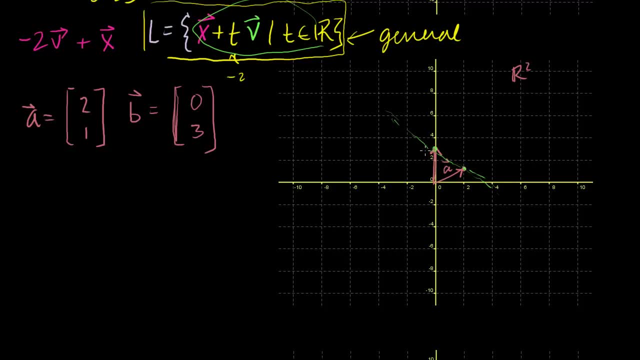 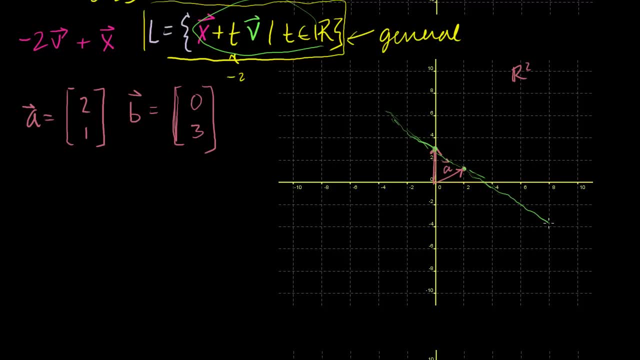 And then instead what we can do is we can say: hey look, this line that goes through both of those points. Or you could almost say that both of those vectors lie on. I guess that's a better. Both of these vectors lie on this line. 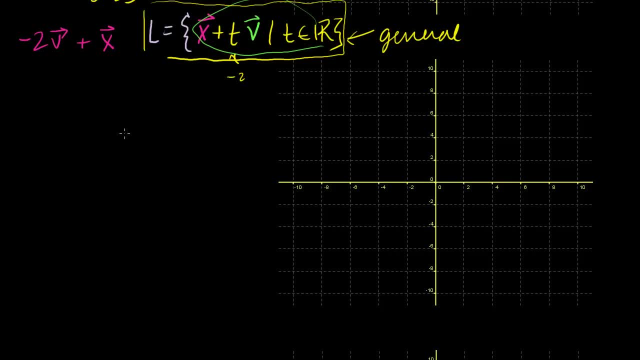 it's the set definition for the line. Let's say we have two vectors. Let's say we have the vector a, which I'll define as 2, 1.. So if I were to draw in standard form, it's 2, 2, 1.. 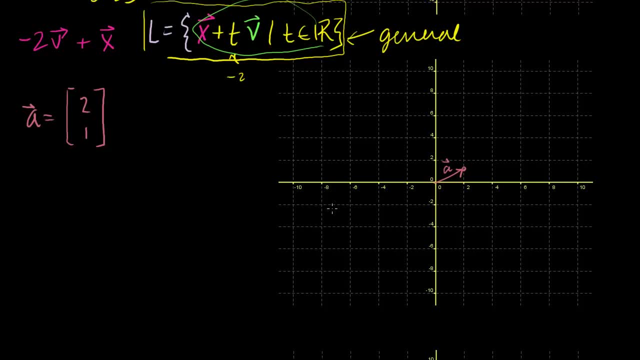 That's my vector a, right there. And let's say I have vector b. Let me define vector b. I'm going to define it as I don't know. let me define it as 0, 3.. So my vector b is 0.. 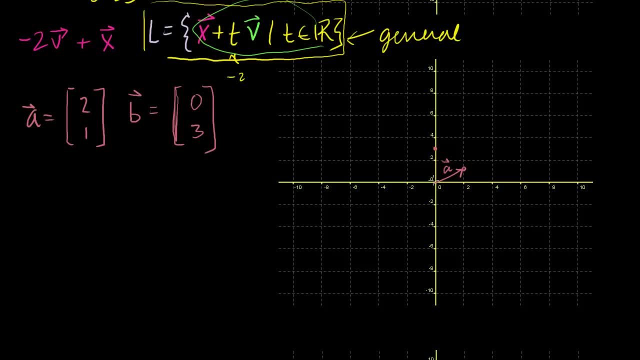 I don't move to the right at all and I go up, So my vector b will look like that. Now I'm going to say that these are position vectors. We draw them in standard form. When you draw them in standard form, their endpoints. 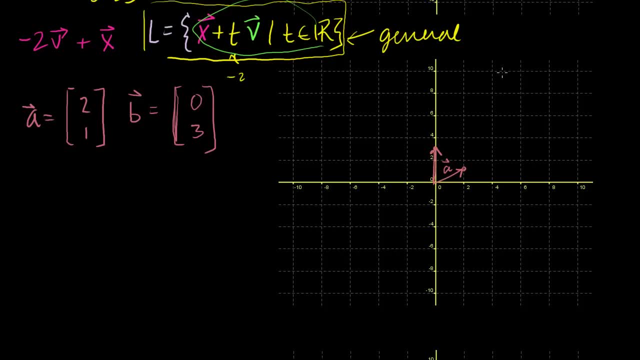 represent some position. So you can almost view these as coordinate points in R2.. This is R2.. I mean, all of these coordinate axes I draw are going to be R2.. Now, what if I asked you give me a parameterization of the? 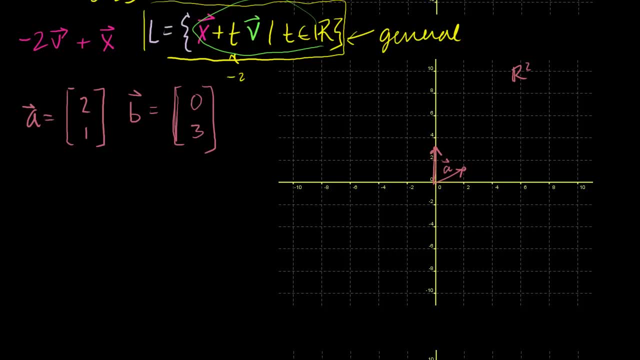 line that goes through these two points. So essentially I want the equation. if you're thinking in Algebra 1 terms, I want the equation for the line that goes through these two points. So the classic way you would have figured out the slope and 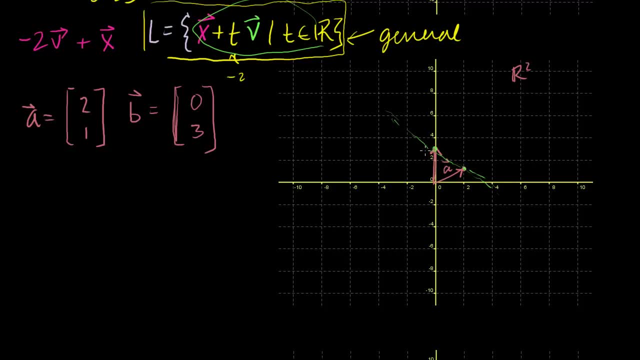 all of that and then you would have substituted back in. But instead what we can do is we can say: hey look, this line that goes through both of those points. you can almost say that both of those vectors lie on. I guess that's a better. 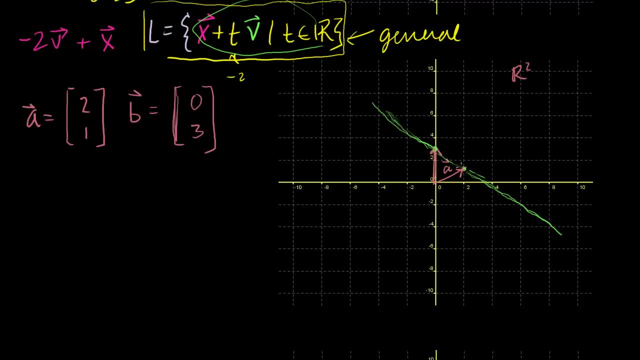 both of these vectors lie on this line. Now, what vector can be represented by that line? Or, even better, what vector, if I take any arbitrary scalar multiple- can represent any other vector on that line? And let me do it this way: 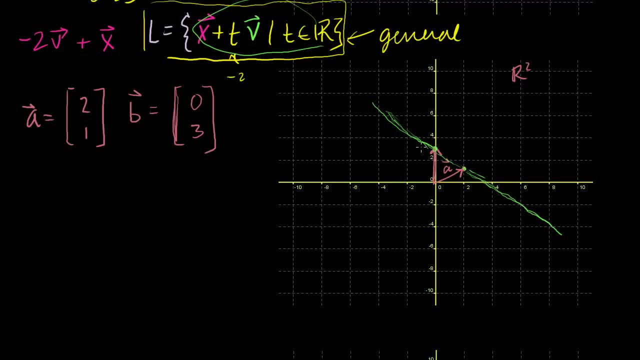 Now, what is the? what vector can be represented by that line? Or, even better, what vector if I take in any arbitrary scale or multiply, it can represent any other vector on that line. What vector if I take any arbitrary scalar revector? not. 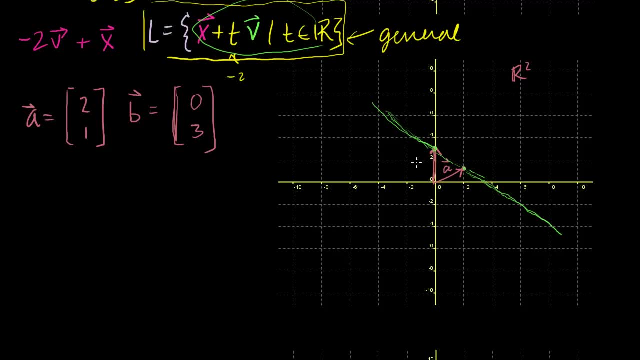 And let me do it this way: What if I were to take: so this is vector b here. what if I were to take b minus a? We learned in- I think it was the previous video- that b minus a- you'll get this vector right here. 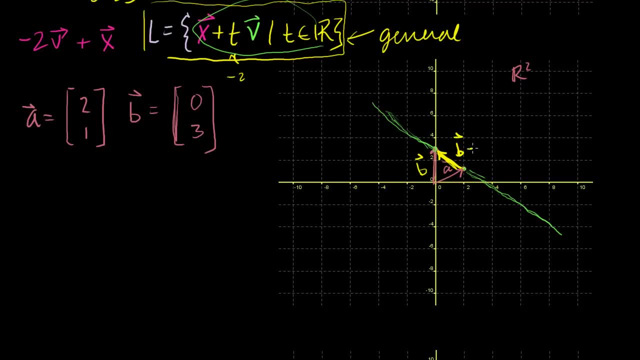 You'll get the difference in the two vectors. This is the vector b minus the vector a, And you just think about it. what do I have to add to a? to get to b, I have to add b minus a. So if I can get the vector b minus a and we know how to do, 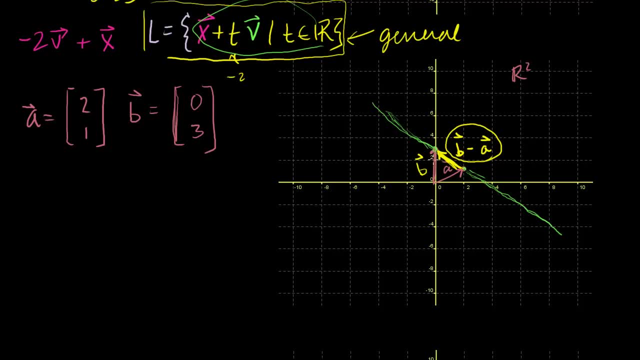 that we just subtract the vectors and then multiply it by any scalar, then we're going to get any point along that line. We have to be careful. So what happens if we take t, so some scalar times our vector times the vectors b minus a? 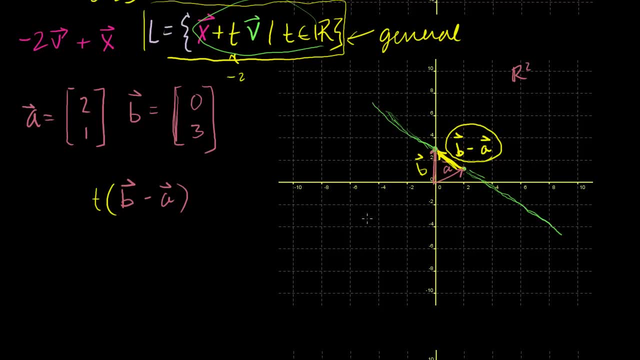 b minus a. What do we get then? So b minus a looks like that, but if we were to draw it in standard form- remember, in standard form- b minus a would look something like this. It would look something like this: 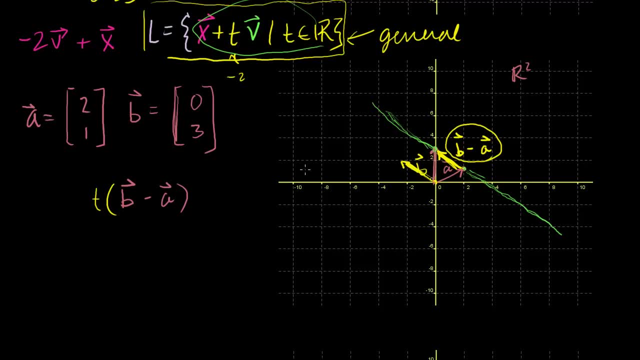 It would start at 0, it would be parallel to this and then from 0, we would draw its endpoint. So if we just multiplied some scalar times b minus a, we would actually just get points or vectors that lie on this line, vectors that lie on that line, right there. 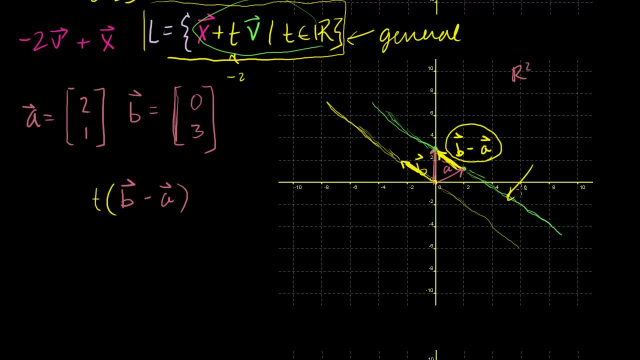 Now, that's not what we set out to do. We wanted to figure out an equation or a parametrization, if you will, of this line or this set. Let's call this set l. So we want to know what that set is equal to. 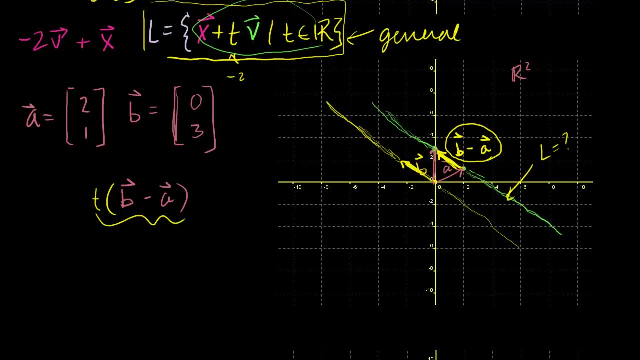 So, in order to get there, we have to start with this, which is this line here, and we have to shift it. And we could shift it either by shifting it straight up. We could add vector b to it, So we could take this line right here and 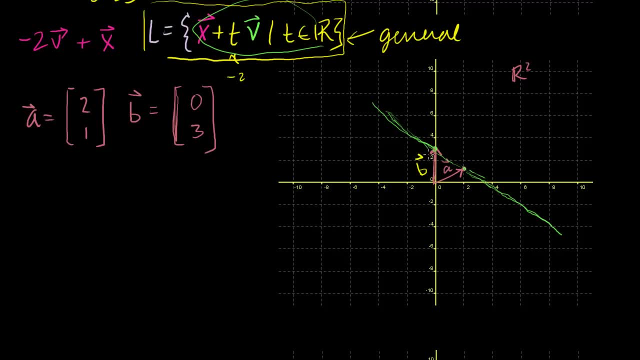 What if I were to take: so this is vector b here. what if I were to take b minus a? We learned in- I think it was the previous video- that b minus a. you'll get this vector right. here You'll get the difference in the two vectors. 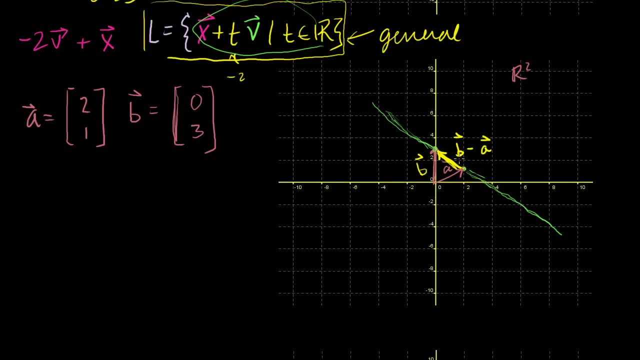 This is the vector b minus the vector a, And you just think about it. what do I have to add to a? to get to b, I have to add b minus a. So if I can get the vector b minus a, and we know how to do that, 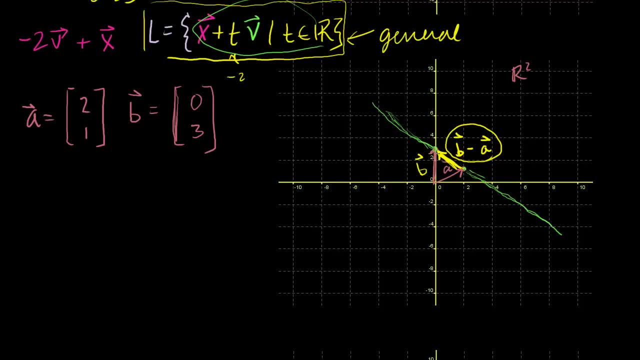 we just suppose subtract the vectors and then multiply it by any scalar, then any scalar, then we're going to get any point along that line. We have to be careful. So what happens if we take t, so some scalar times our vector times the vectors b minus a? 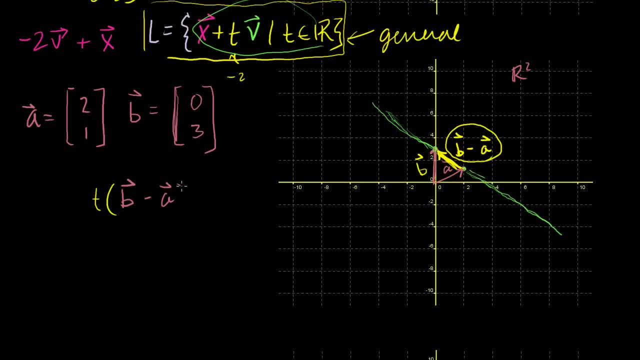 b minus a. What do we get then? So b minus a looks like that, but if we were to draw it in standard form- remember, in standard form- b minus a would look something like this. It would look something like this: 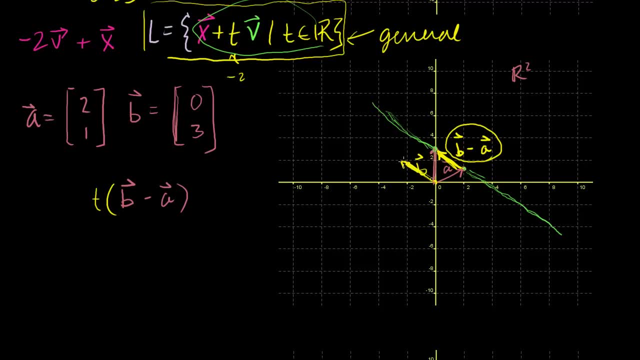 Right, It would start at zero, it would be parallel to this, and then from zero we would draw its end point. So if we just multiplied some scalar times b minus a, we would actually just get points or vectors that lie on this line. 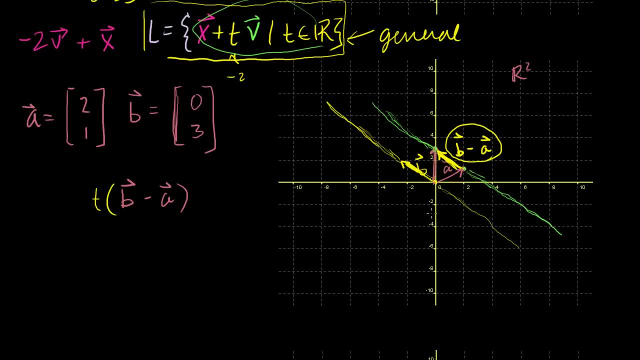 Vectors that lie on that line right there. Now, that's not what we set out to do. We wanted to figure out an equation or a parametrization, if you will, of this line or this set. Let's call this set L. 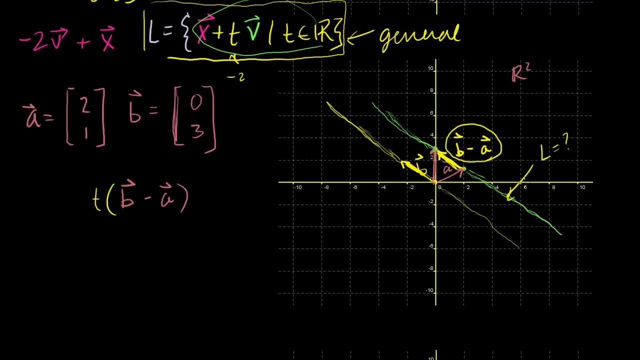 So we want to know what that set is equal to. So, in order to get there, we have to start with this: which is this line, which is this line here, and we have to shift it. And we could shift it either by shifting it straight up. 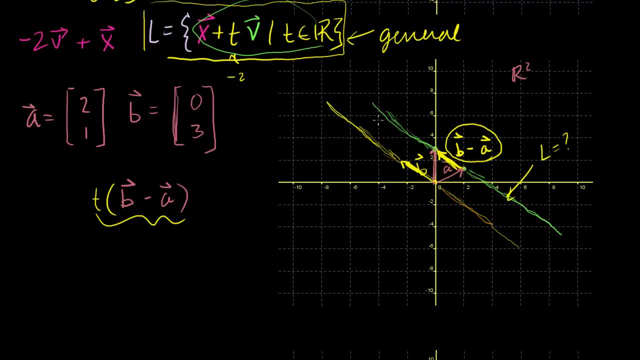 we could add vector b to it. so we could take this line right here and add vector b to it, and so any point on here would have its corresponding point there. So when you add vector b, it essentially shifts it up. That would work. 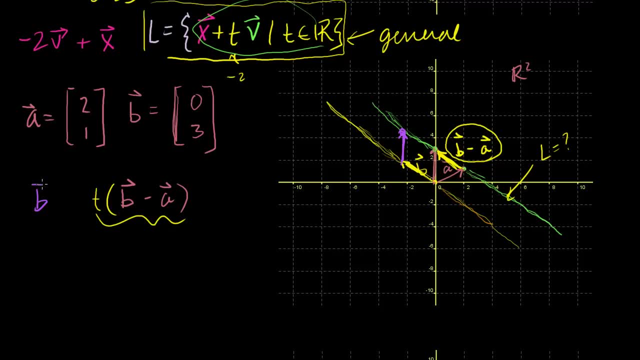 So we could say we could add vector b to it. and now all of these points, for any arbitrary t is a member of the real numbers will lie on this green line. Or the other option we could have done is we could have added vector a. 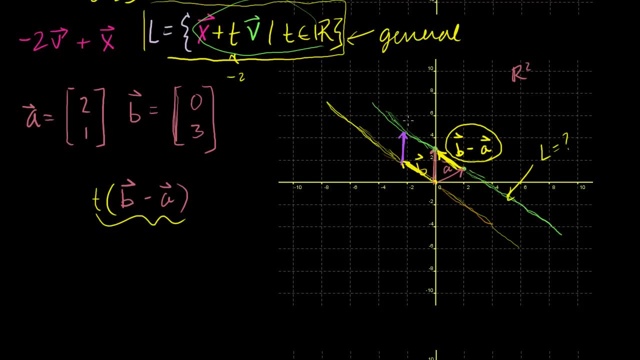 add vector b to it, And so any point on here would have its corresponding point there. So when you add vector b, it essentially shifts it up. That would work. So we could say: we could add vector b to it. And now all of these points, for any arbitrary t is a. 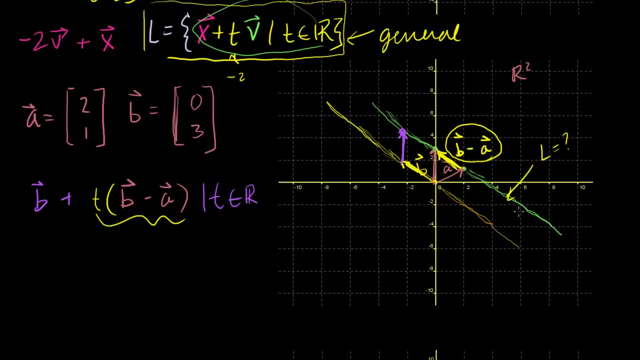 member of the real numbers will lie on this green line Or the other option we could have done is we could have added vector a. Vector a would have taken any arbitrary point here and shifted it. that way You would be adding vector a to it. 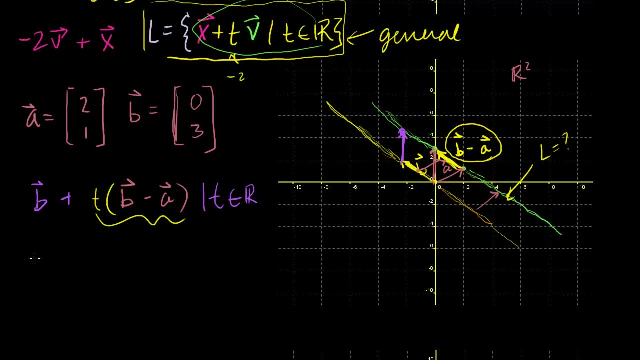 But either way you're going to get to the green line that we cared about. So you could have also defined it as the set of vector a Plus this line essentially t times vector b minus a, Where t is a member of the reals. 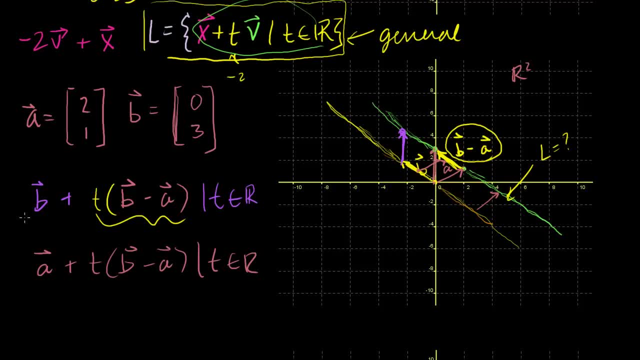 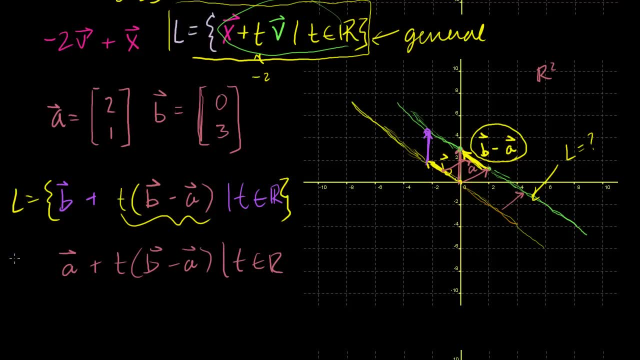 Now all of this. so my definition of my line could be either of these things. The definition of my line could be this set, Or it could be this set, And all of this seems all very abstract, But when you actually deal with the numbers, it actually 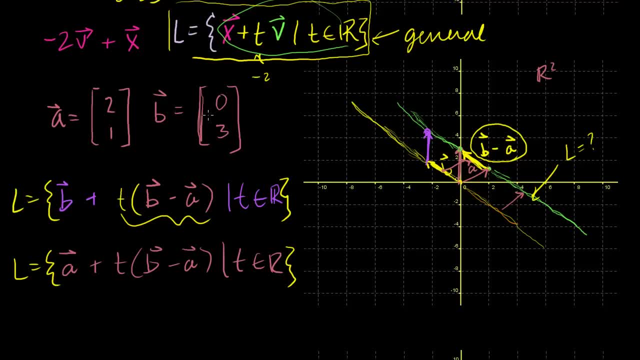 becomes very simple. It becomes arguably simpler than what we did in Algebra 1.. So this l for this particular case of a and b. let's figure it out. My line is equal to- let me just use the first example: It's vector b. 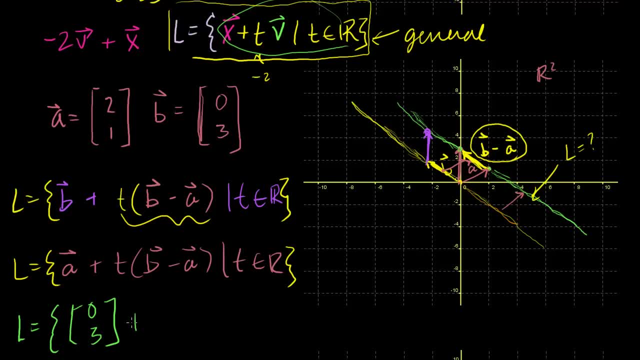 So it's the vector 0, 3 plus t times the vector b minus a. What's b minus a? 0 minus 2 is minus 2.. 3 minus 1 is 2. 4. t. t is a member of the reals. 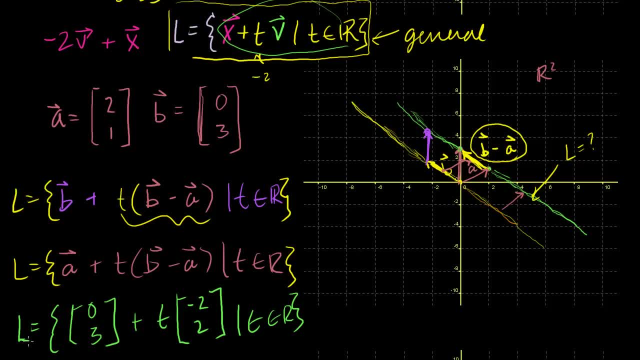 Now, if this still seems kind of like a convoluted set definition for you, I could write it in terms that you might recognize better. If we want to plot points, if we call this the y-axis and we call this the x-axis and if we call this the x. 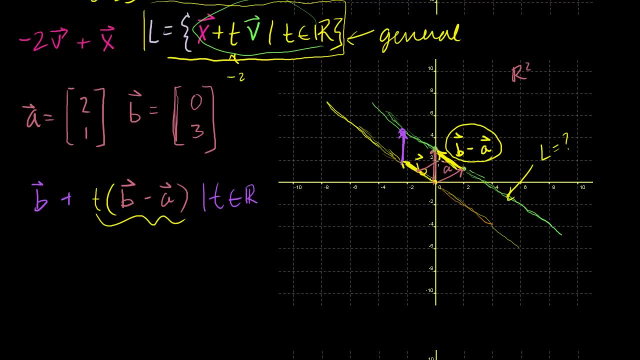 Vector a would have taken any arbitrary point here and shifted it. that way You would be adding vector a to it, But either way you're going to get to the green line that we cared about, So you could have also defined it as a vector a plus this line. essentially, 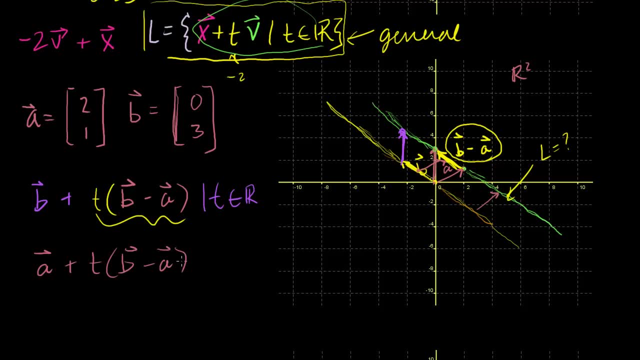 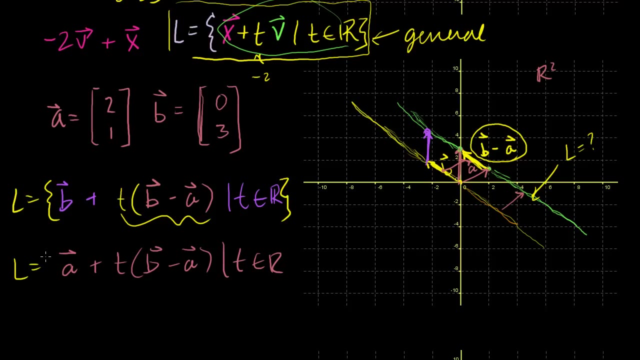 t times vector b minus a, where t is a member of the reals. Now all of this. so my definition of my line could be either of these things. The definition of my line could be this set, or it could be this set: 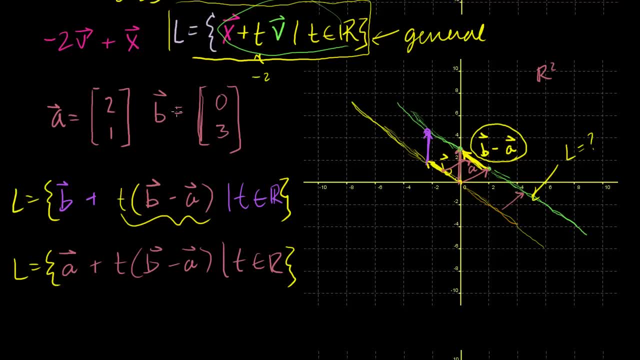 And all of this seems all very abstract, but when you actually deal with the numbers it actually becomes very simple. It becomes arguably simpler than what we did in Algebra 1.. So this l for this particular case of a and b. let's figure it out. 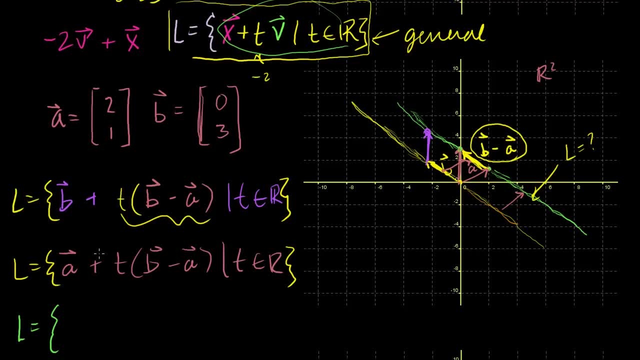 My line is equal to- let me just use the first example. It's vector b, so it's the vector 0, 3 plus t times the vector b minus a. What's b minus a? 0 minus 2 is minus 2.. 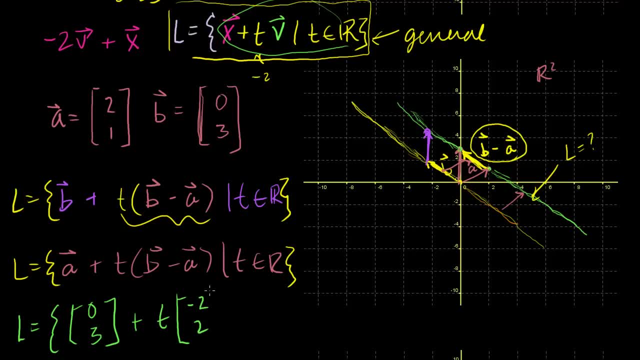 3 minus 1 is 2.. 4t is a member of the reals. Now, if this still seems kind of like a convoluted set definition for you, I could write it in terms that you might recognize better If we want to plot points. 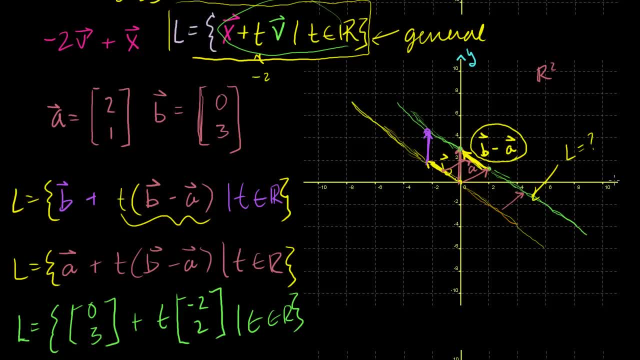 if we call this the y-axis and we call this the x-axis, and if we call this the x-coordinate, or maybe more properly that the x-coordinate, and call this the y-coordinate, then we could set up an equation here. 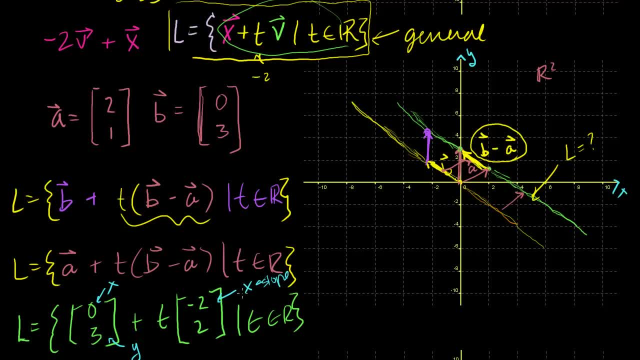 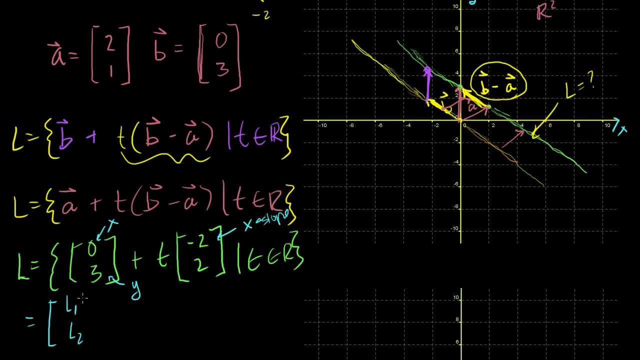 This actually is the x-slope, This is the x-coordinate and that's the y-coordinate, Or actually even better, whatever. actually, let me be very careful there. this is always going to end up becoming some vector l1, l2.. 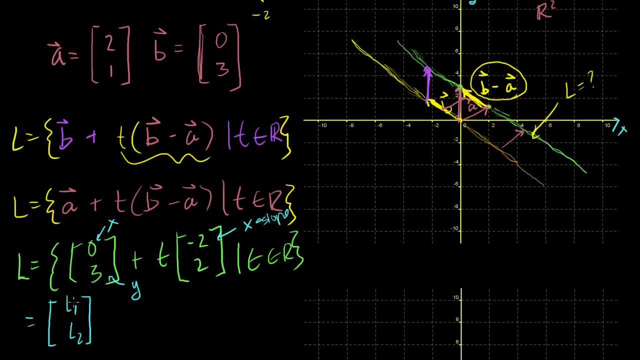 This is a set of vectors and any member of the set is going to look something like this. This could be li, This is the x-coordinate and this is the y-coordinate. And just to get this coordinate, and just to get this in a form that you recognize, 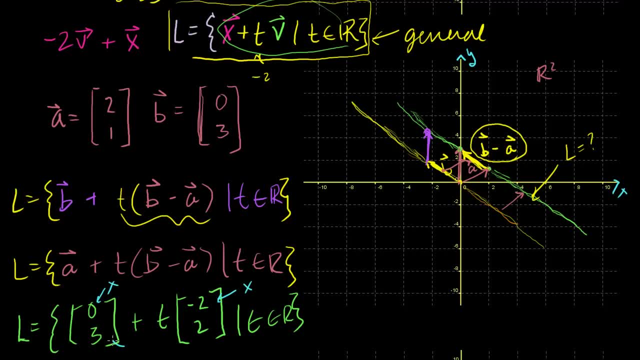 coordinate, or maybe more properly that the x coordinate and call this the y coordinate. then we can set up an equation here. This actually is the x-slope, With respect. Well, I don't want to. This is the x-coordinate and that's the y-coordinate. 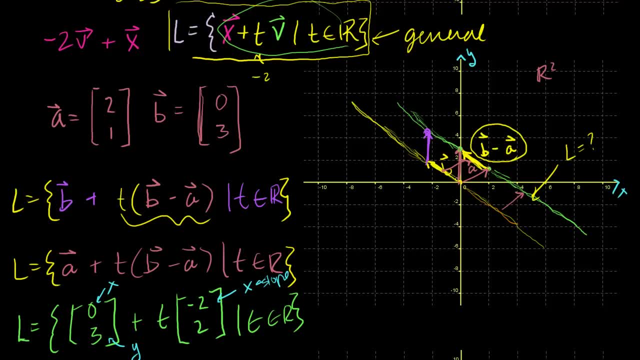 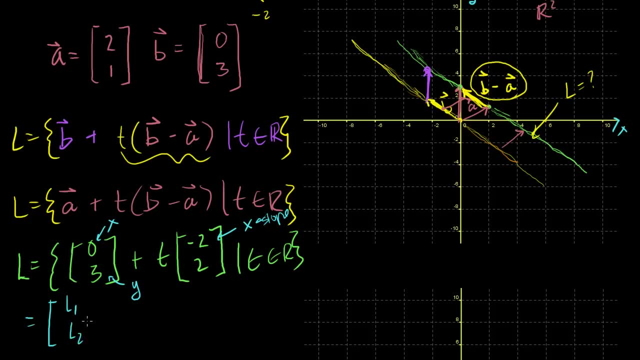 Or actually even better, whatever. Actually, let me be very careful there. This is always going to end up becoming some vector l1,, l2.. This is a set of vectors, and any member of the set is going to look something like this: 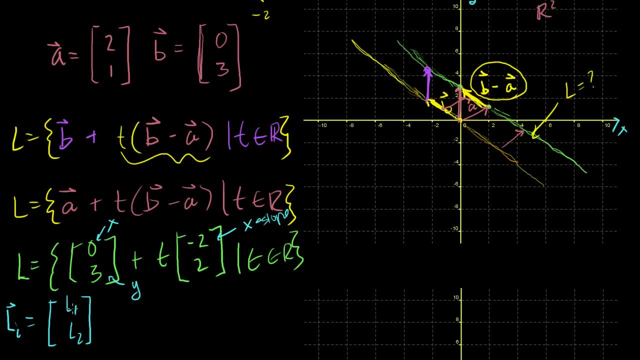 So this could be li. So this is the x-coordinate and this is the y-coordinate, And just to get this coordinate and just to get this in a form that you recognize, so we're saying that l is a set of this vector x plus t times this vector b. 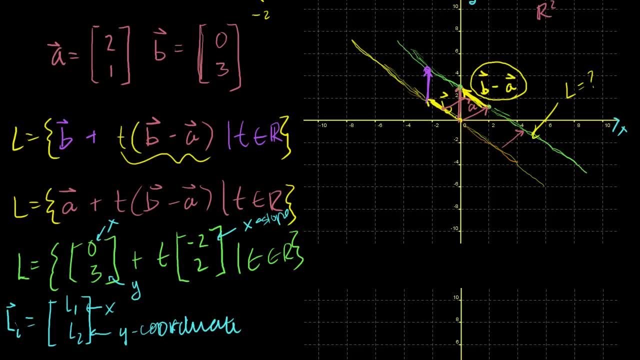 minus a. here, If we wanted to write it in kind of a parametric form, we can say: since this is what determines our x-coordinate, we would say that x is equal to 0 plus t times minus 2, or minus 2 times t. 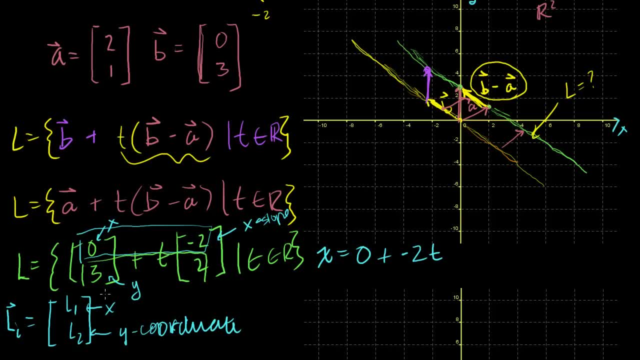 And then we can say that y- since this is what determines our y-coordinate y- is equal to 3 plus t times 2, plus 2t. So we could have rewritten that first equation as just x is equal to minus 2t and y is equal to 2t plus 3.. 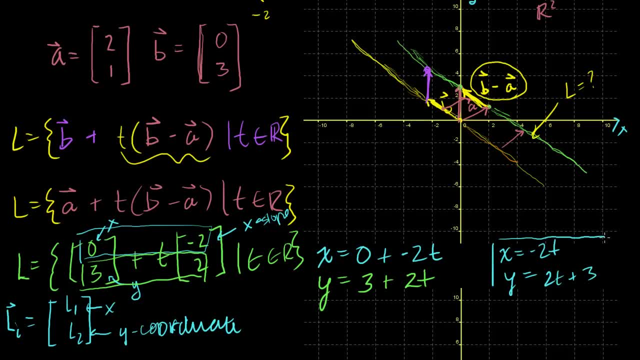 So if you watch the videos on parametric equations, this is just a traditional parametric definition of this line, This line right there Now you might have still viewed this as Sal. this was a waste of time. this was convoluted. you had to define. 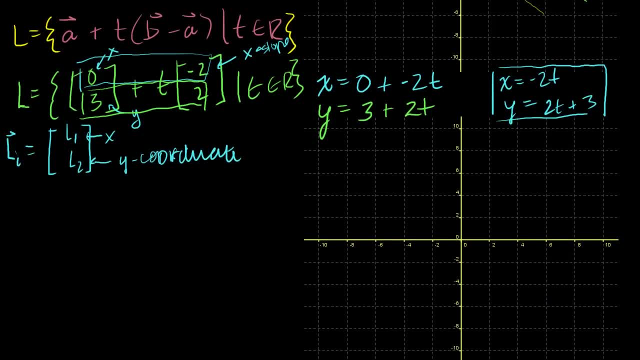 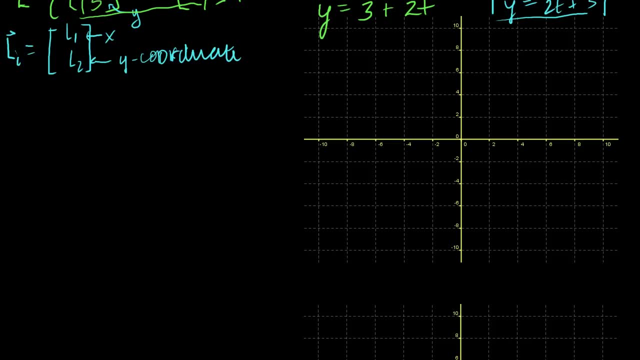 these sets and all of that. But now I'm going to show you something that you probably- well, unless you've done this before- I guess that's true of anything, but you probably haven't seen in your traditional algebra class. Let's say I have two points. 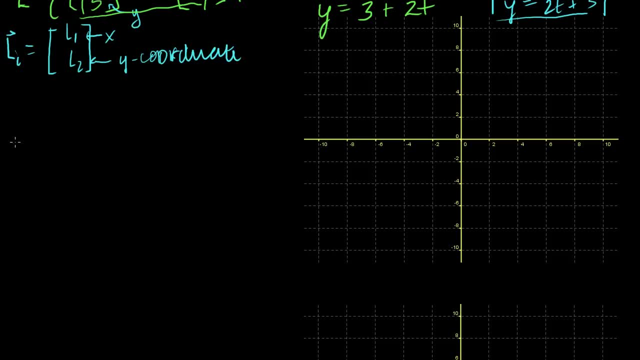 And now I'm going to deal in three dimensions. So let's say I have one vector- I'll just call it point 1, because these are position vectors, so let's call it position 1.. And it's the point. This is in three dimensions. 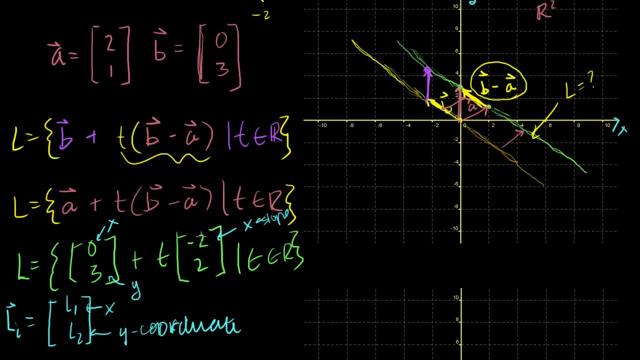 so we're saying that l is a set of, you know, this vector x plus t times this vector t, times this vector b minus a. here, If we wanted to write it in kind of a parametric form, we can say: since this is what determines our x-coordinate: 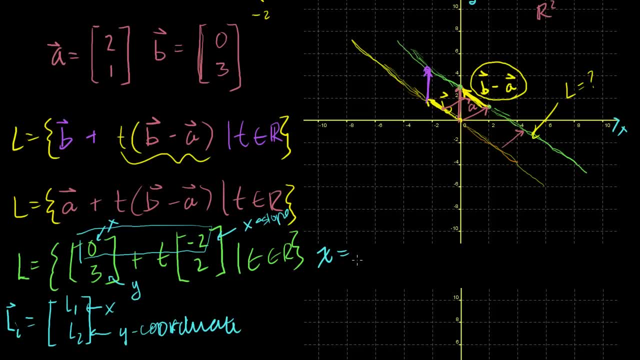 we would say that x is equal to 0 plus t times minus 2,, or minus 2, minus 2 times t, And then we can say that y- since this is what determines our y-coordinate y- is equal to 3 plus t times 2,. 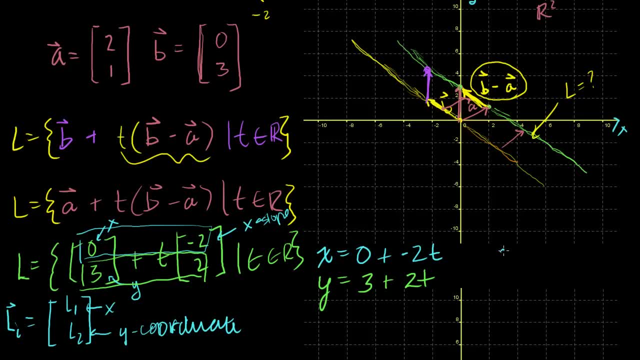 plus 2t. So we could have rewritten that first equation, as just x is equal to minus 2t and y is equal to 2t plus 3.. So if you watch the videos on parametric equations, this is just a traditional. 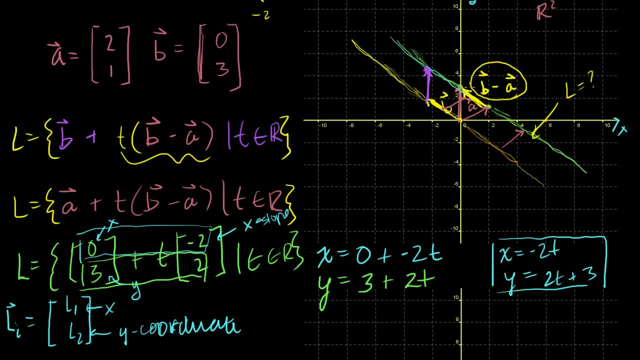 parametric definition of this line, this line, right there Now. you might have still viewed this as Sal. this was a waste of time, this was convoluted, you had to define these sets and all of that, but now I'm going to show you something. 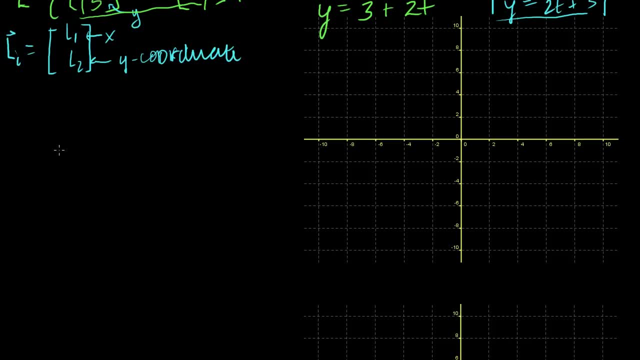 that you probably. well, unless you've done this before, I guess that's true of anything, but you probably haven't seen it in your traditional algebra class. Let's say I have two points and now I'm going to deal in three dimensions. 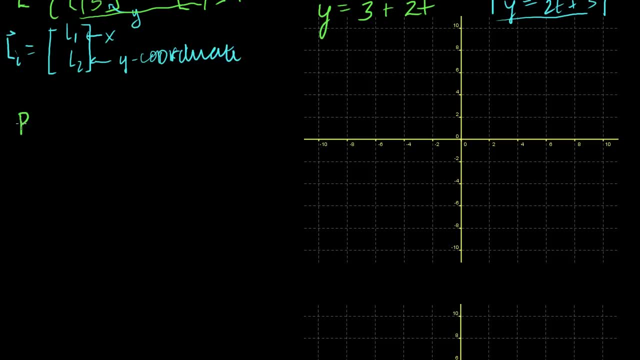 So let's say I have one vector. I'll just call it 0.1. Because these are position vectors, so let's call it position 1.. And this is the point. this is in three dimensions. Let's make up some numbers. 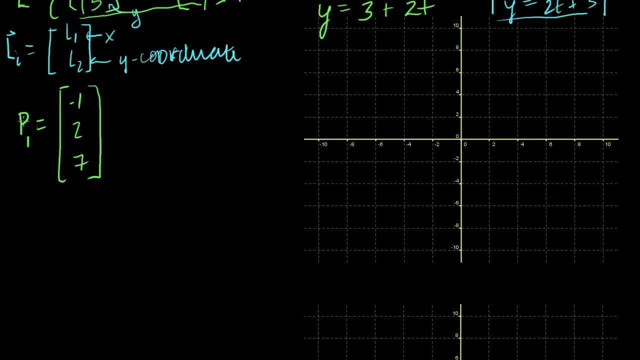 negative: 1,, 2, 7.. Let's say I have 0.2.. And once again this is in three dimensions, so you have to specify three coordinates. This could be the x, the y and the z coordinate. 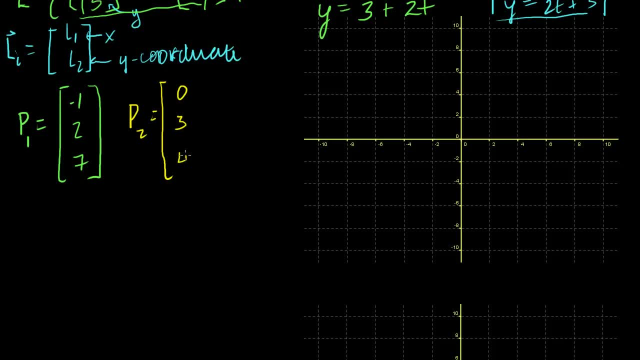 0.2, I don't know. let's make it 0,, 3, and 4.. Now what if I wanted to find the equation of the line that passes through these two points in R3?? So this is in R3.. 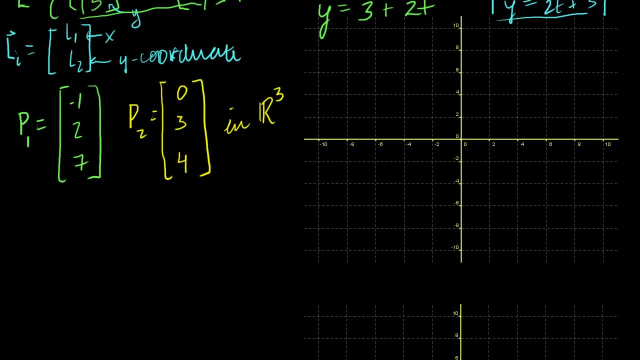 Well, I just said that, the equation of this line, so I'll just call that, or the set of this line. let me just call this. you know, L. It's going to be equal to. we could just pick one of these guys. 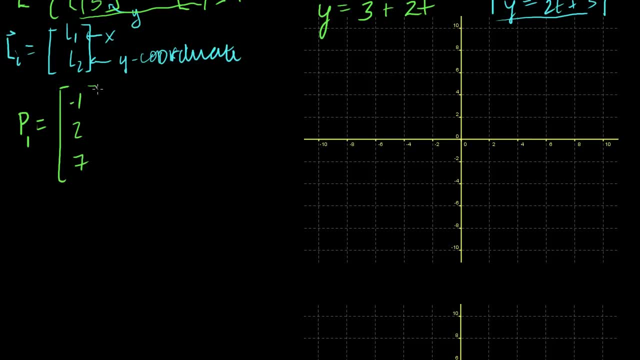 Let's make up some numbers, Negative: 1,, 2,, 7. Let's say I have point 2. And once again this is in three dimensions. So you have to specify three coordinates. This could be the x, the y and the z coordinate. 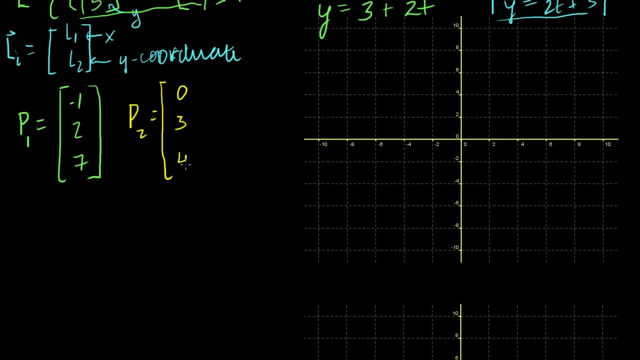 Point 2, I don't know. let's make it 0,, 3, and 4.. Now what if I wanted to find the equation of the line that passes through these two points in R3?? So this is in R3.. 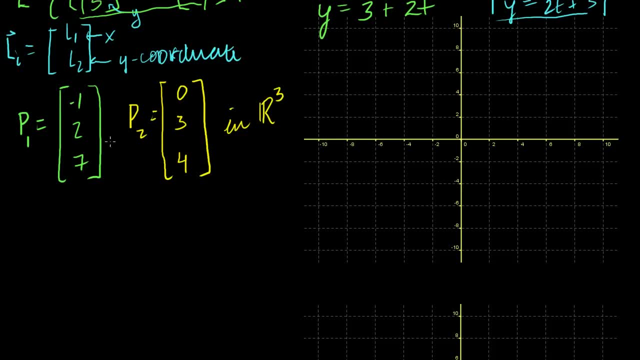 Well, I just said that the equation of this line, or the set of this line- let me just call this l- it's going to be equal to. we could just pick one of these guys: It could be p1, the vector p1.. 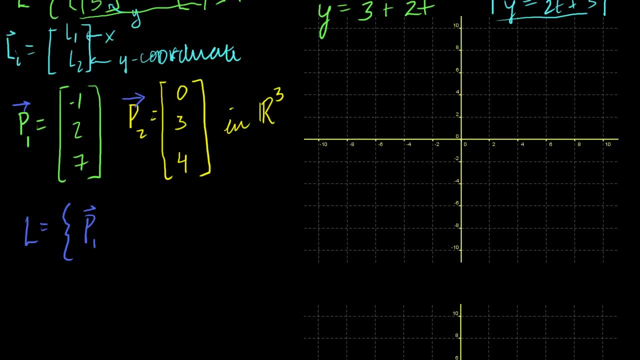 These are all vectors, Be careful here. The vector p1 plus some random parameter t. this t could be time, like you learned when you first learned parametric equations. Times the difference of the two vectors, Times p1, and it doesn't matter what order you take it. 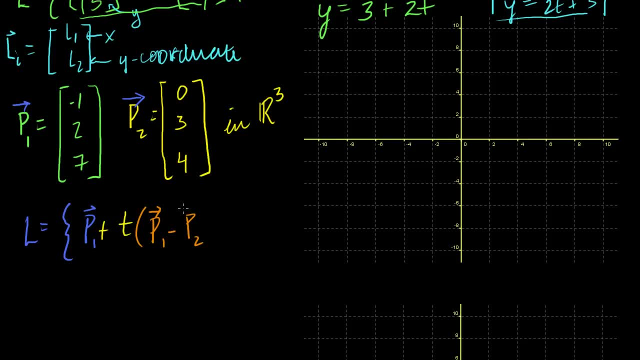 So that's a nice thing too: p1 minus p2.. It could be p2 minus p1, because this can take on any positive or negative value where t is a member of the real numbers. So let's apply it to these numbers. 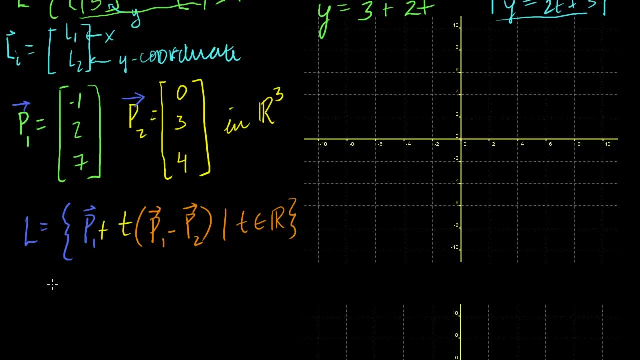 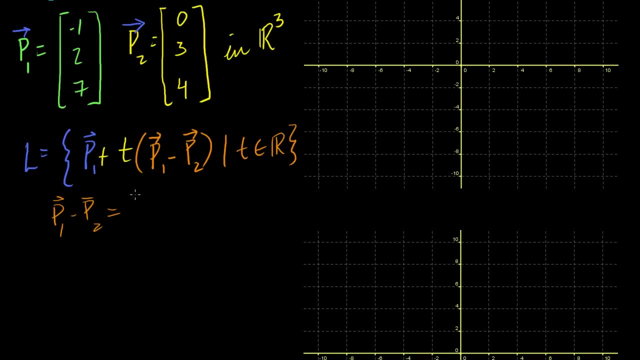 Let's apply it right here. What is p1 minus p2?? p1 minus p2 is 0.. Is equal to. let me get some space here: p1 minus p2 is equal minus 1 minus 0, is minus 1.. 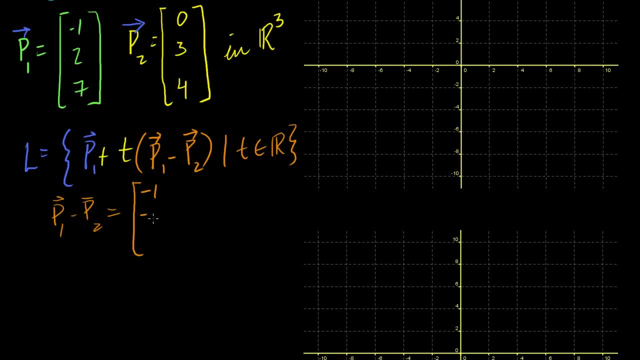 2 minus 3 is minus 1.. 7 minus 4 is 3.. So that thing is that vector, And so our line can be described as a set of vectors that, if you were to plot it in standard position, it would be. 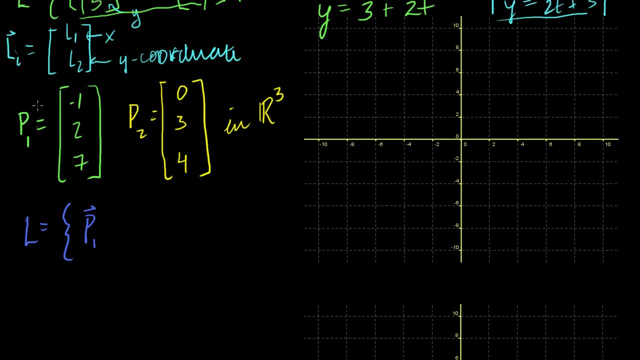 It's going to be. it could be P1, the vector P1, these are all vectors, be careful here. The vector P1 plus some random parameter T. this T could be time, like you learn when you first learn parametric equations. 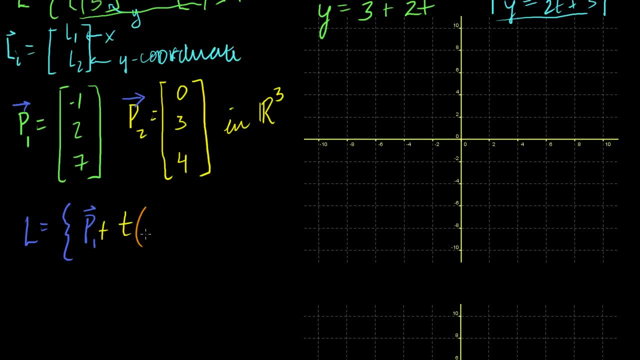 times the difference of the two vectors, times P1,, and it doesn't matter what order you take it, so that's a nice thing too: P1 minus P2.. It could be P2 minus P1,, and then this, you know: 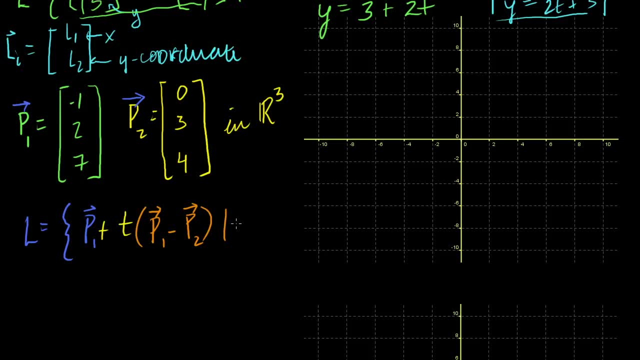 because this can take on any positive or negative value where T is a member of the real numbers. So let's apply it to these numbers, Let's apply it right here. What is P1 minus P2?? P1 minus P2 is equal to. 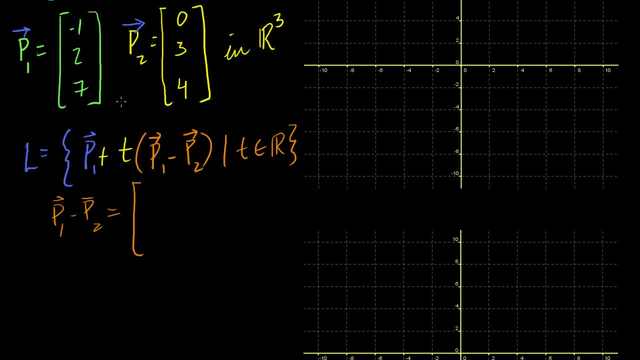 let me get some space here. P1 minus P2 is equal minus 1 minus 0 is minus 1,. 2 minus 3 is minus 1,. 7 minus 4 is 3.. So that thing is that vector. 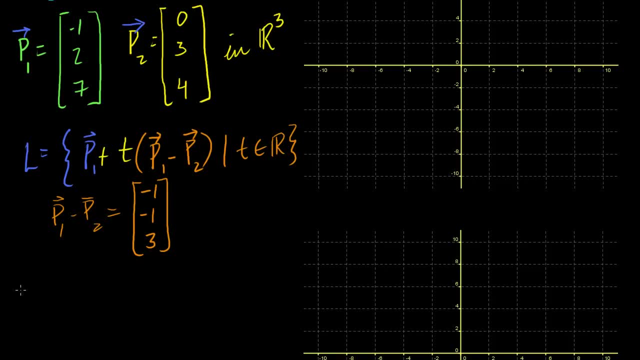 and so our line can be described as a set of vectors that, if you were to plot it in standard position, it would be this set of position vectors. It would be P1, it would be- let me do that in green- it would be minus 1,, 2,, 7,. 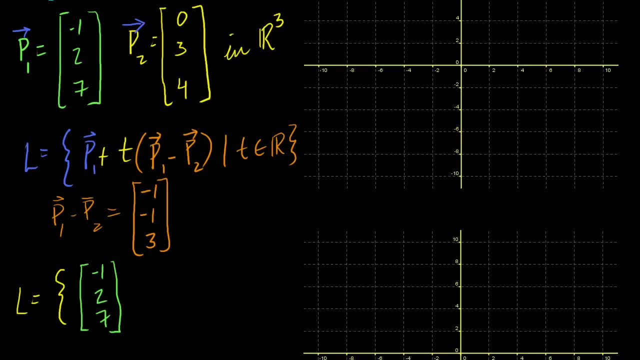 I could have put P2 there just as easily: plus T times minus 1,, minus 1, 3,, which is another set of vectors. So we have this set of vectors. you just know, it's a set of vectors. Now, if you had, 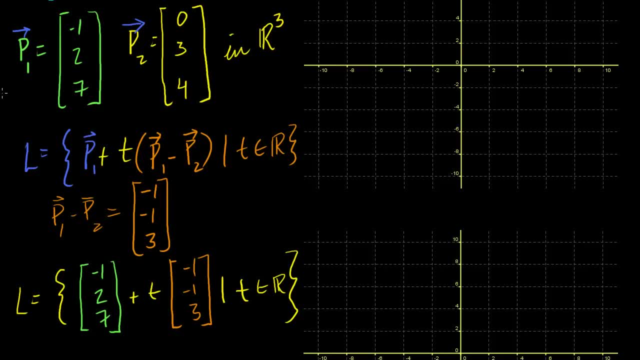 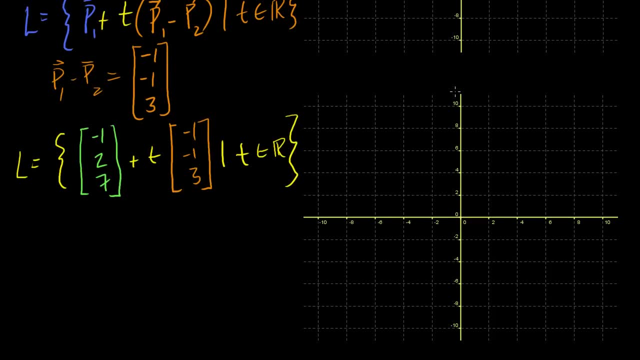 let me move the counter to the left here. So if I had a set of vectors and you had a set of vectors, P1 minus T times 1, minus 1 is minus 1,. 2 minus P2 minus 2 is minus 1,. 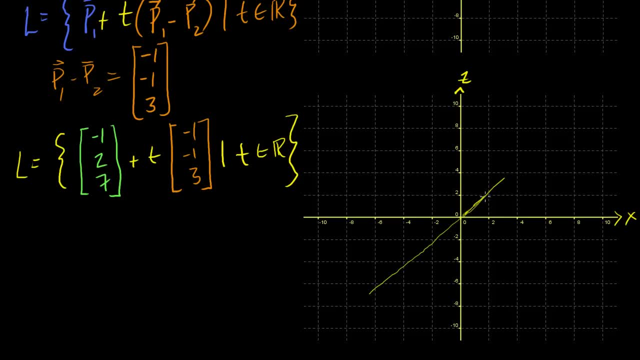 so that's the set of vectors into our board like this. So the y-axis comes out like that. So what you can view, this, and actually I probably won't graph- so the determinant for the x-coordinate, just our convention, is going to be this term, right here. 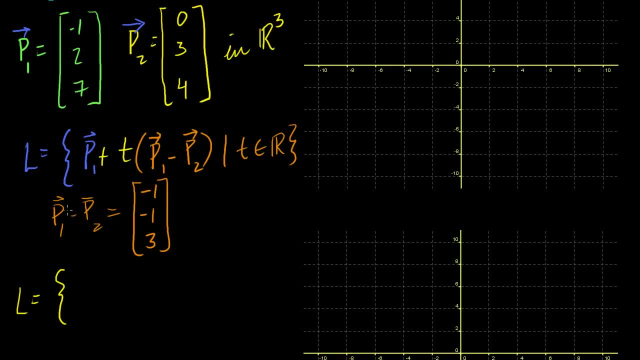 this set of position vectors. So it would be p1, it would be- let me do that in green- It would be minus 1, 2, 7.. I could have put p2 there just as easily. Plus t times minus 1, minus 1, 3.. 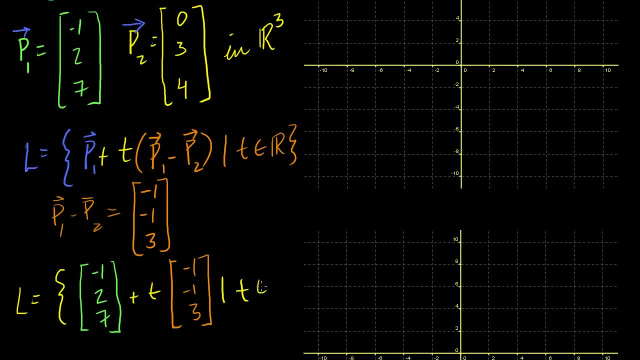 Where or such, that t is a member of the real numbers. Now, this also might not be satisfying for you. You're like gee. Now how do I plot this in three dimensions? Where is my x, y's and z's? 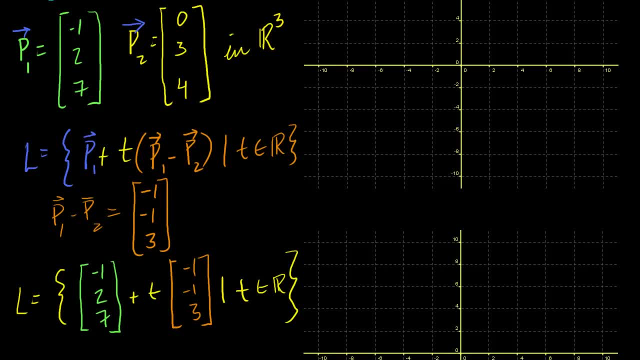 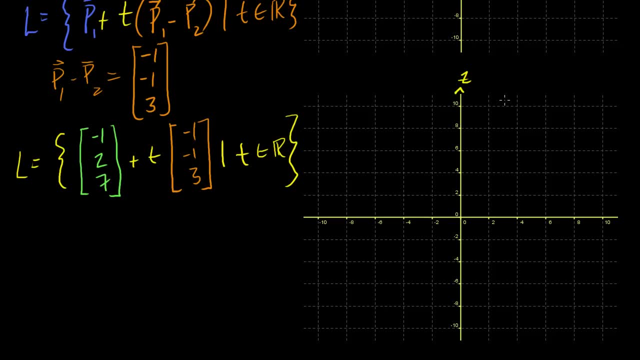 And if you want to care about x, y's and z's, let's say that this is. let me go down here. Let's say that this is the z-axis, This is the x-axis, And let's say the y-axis. 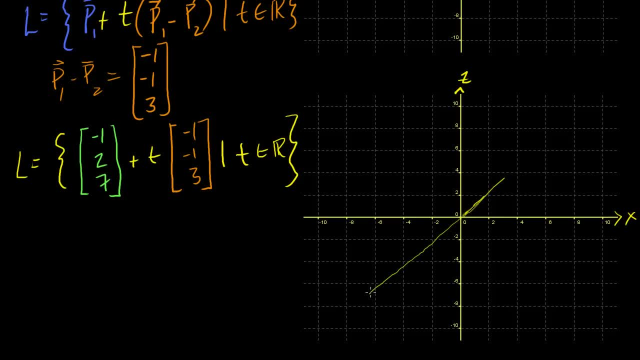 It kind of goes into our board like this, So the y-axis comes out like that. So what you can view this, and actually I probably won't graph- so the determinant for the x-coordinate, just our convention, is going to be this term, right here. 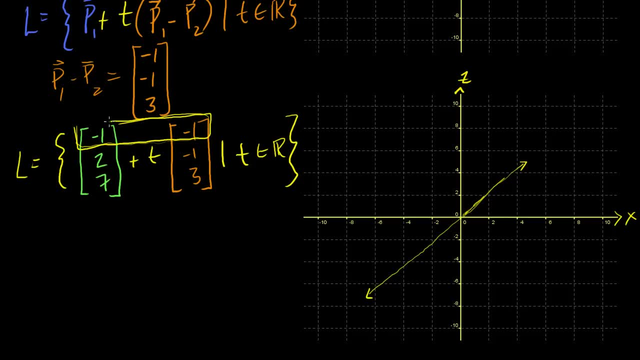 So we can write that x. let me write that down. So that term is going to determine our x-coordinate. So we can write that x is equal to minus 1, be careful with the colors: minus 1 plus minus 1 times t. 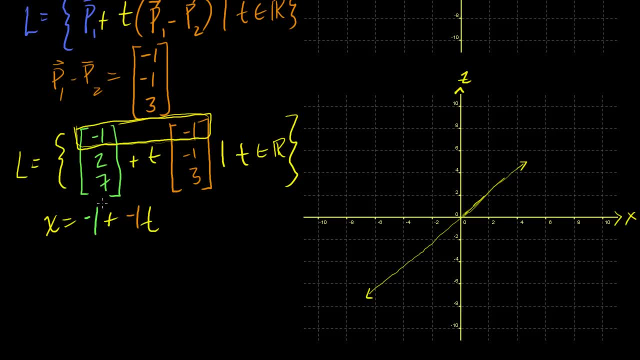 Plus minus 1 times t. That's our x-coordinate, That's our x-coordinate, That's our x-coordinate. Now our y-coordinate, Now our y-coordinate, Now our y-coordinate coordinate is going to be determined by this part of our 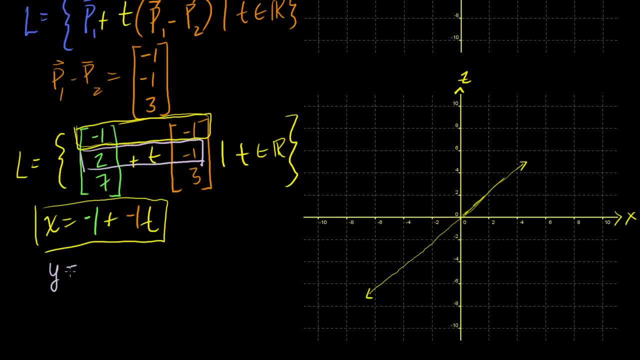 vector addition, because these are the y-coordinates. So we could say that our y-coordinate is equal to- I'll just write it like this- 2 plus minus 1 times t, And then, finally, our z-coordinate is determined by that there. 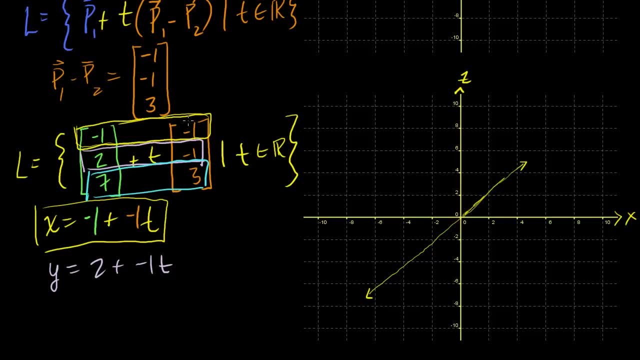 The t shows up because it's t times 3, or I could just put this t into all of this. So the z-coordinate is equal to 7 plus t times 3, or I could say plus 3t, And just like that we have three parametric equations. 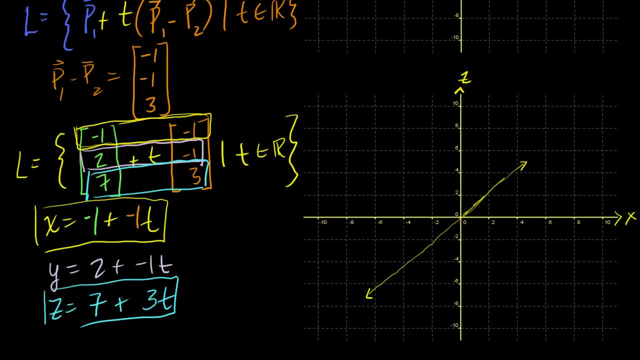 And when we did it in R2, I did a parametric equation, but we learned in Algebra 1 you could just have a regular y in terms of x. You don't have to have a parametric equation, But when you're dealing in R3, the only way to define a line 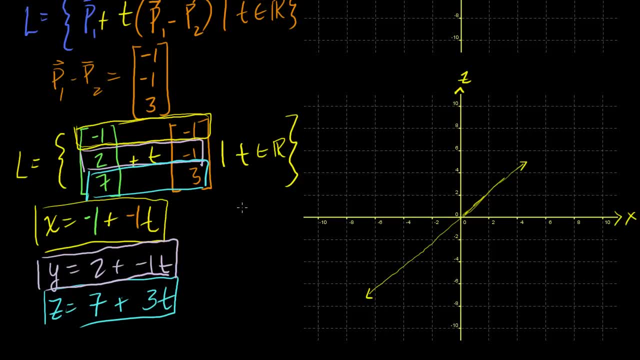 is to have a parametric equation. If you have just an equation with x's, y's and z's, if I just have x plus y plus z, is equal to some number. this is not a line And we'll talk more about this in R3.. 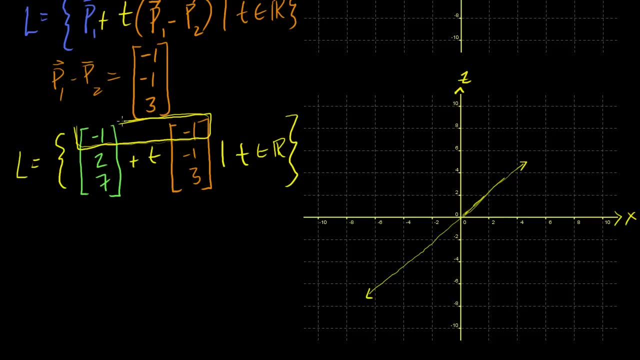 So we can write that x. let me write that down. So that term is going to determine our x-coordinate. So we can write that x is equal to minus 1, be careful with the colors: minus 1 plus minus 1 times t. 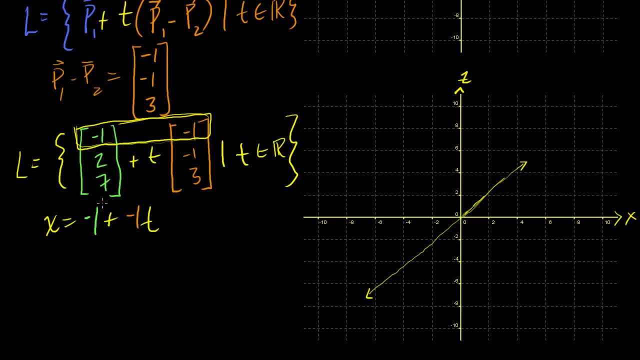 Plus minus 1 times t. That's our x-coordinate. Now our y-coordinate is going to be determined by this part of our vector addition, because these are the y-coordinates. So we could say that our y-coordinate is equal to I'll. 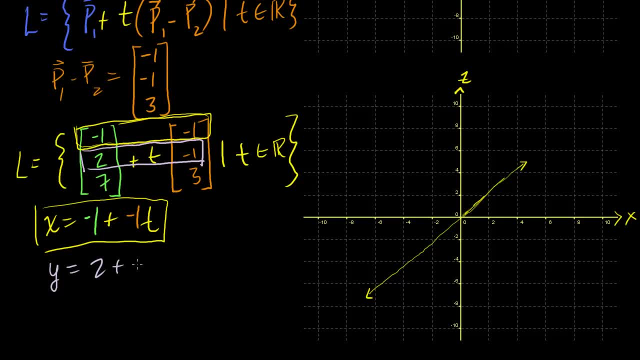 just write it like this: 2 plus minus 1 times t, And then, finally, Our z-coordinate is determined by that there and the t shows up because it's t times 3, or I could just put this t into all of this. 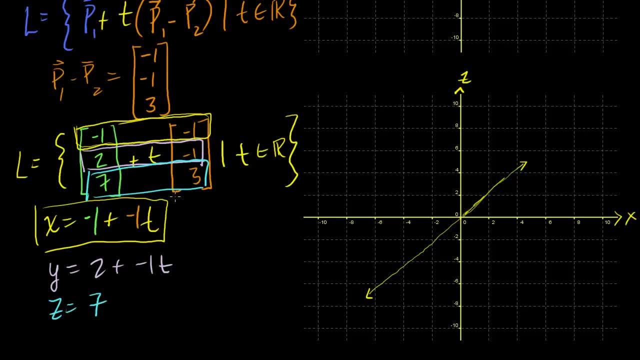 So the z-coordinate is equal to 7 plus t times 3,, or I could say plus 3t, And just like that we have three parametric equations. And when we did it in R2, I did a parametric equation but we 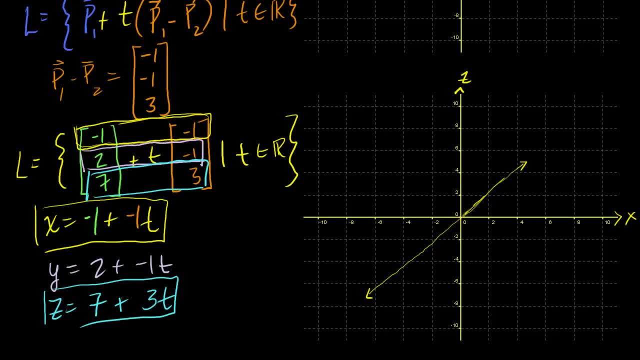 learned in Algebra 1, you could just have a regular y in terms of x. you don't have to have a parametric equation. But when you're dealing in R3, the only way to define a line is to have a parametric equation. 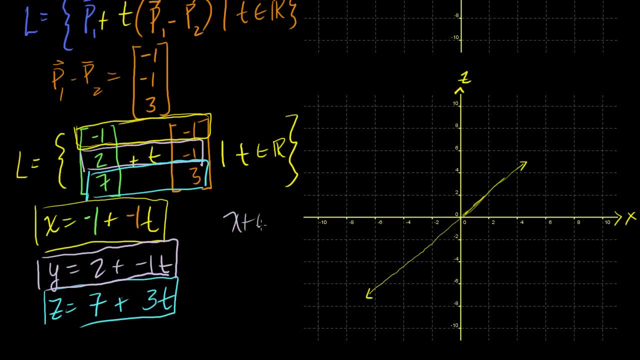 If you have just an equation with x's, y's and z's, if I just have x plus y plus z is equal to some number. this is not a line. We'll talk more about this in R3.. This is a plane. 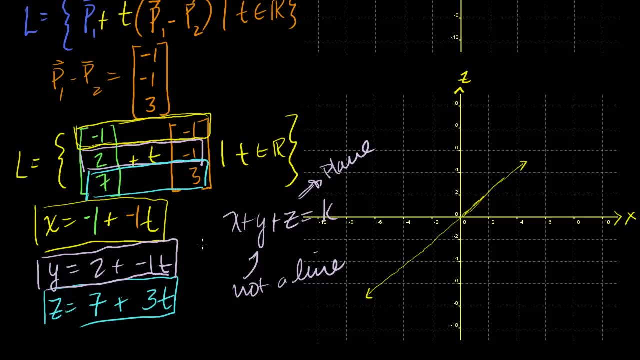 The only way to define a line or a curve in three dimensions. if I wanted to describe the path of a fly in three dimensions, it has to be a parametric equation. Or if I were to shoot a bullet in three dimensions and it goes in a straight line, it has to be a 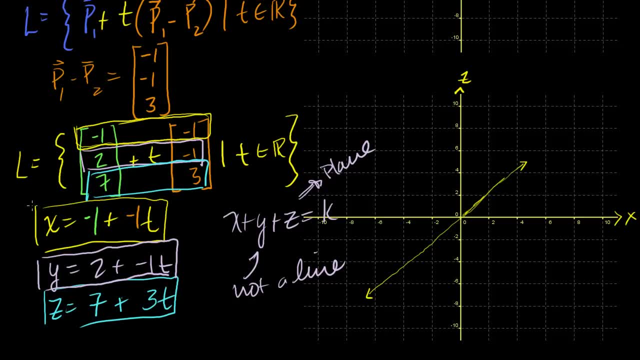 parametric equation. So these, I guess we call it, these are the equations of a line in three dimensions. So hopefully you found that interesting And I think this will be the first video where you have an appreciation that linear algebra can solve problems, or